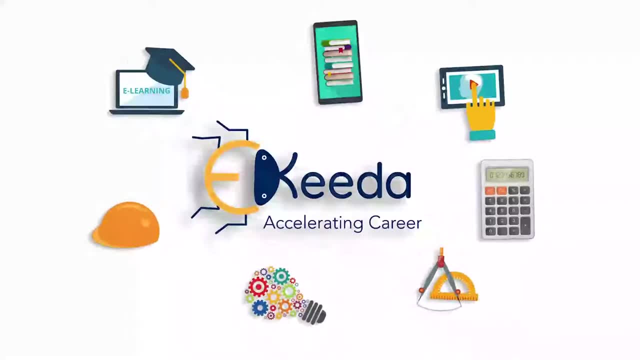 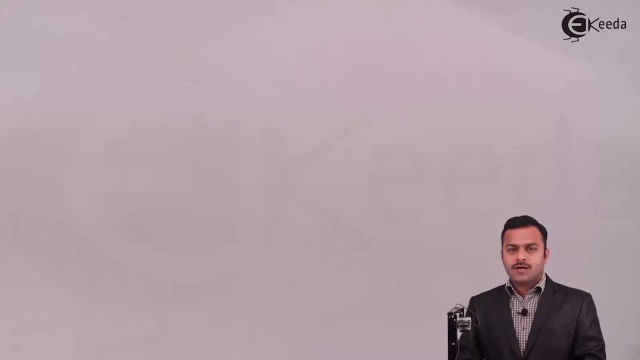 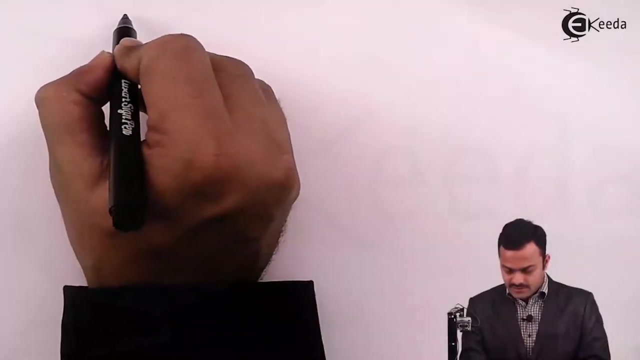 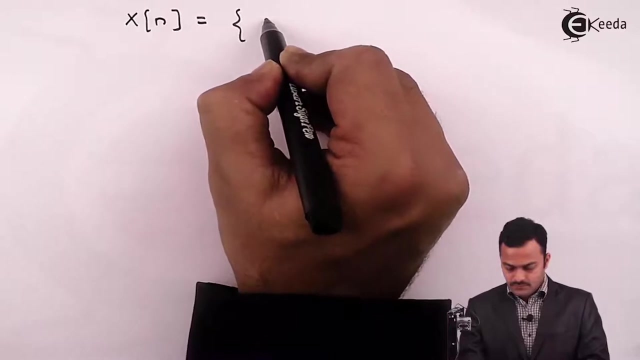 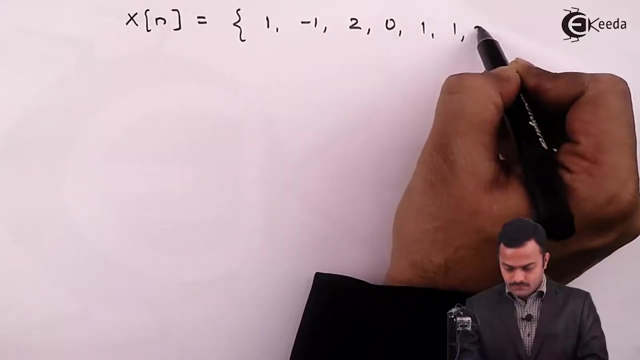 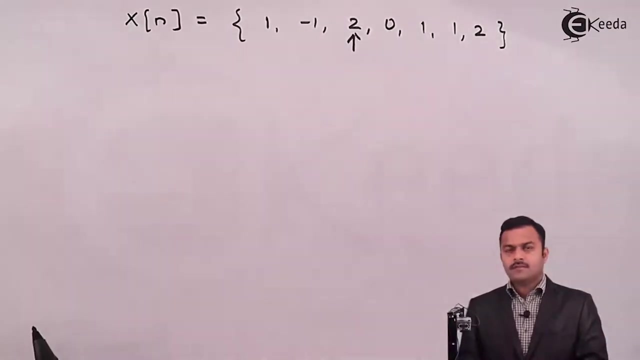 In this video we are going to see basic signal operations like time reversal, time shifting, time scaling for a discrete time signal. So X of n is a discrete time signal given as n equal to 0.. At origin is this. So this is an indication of an origin. means what? 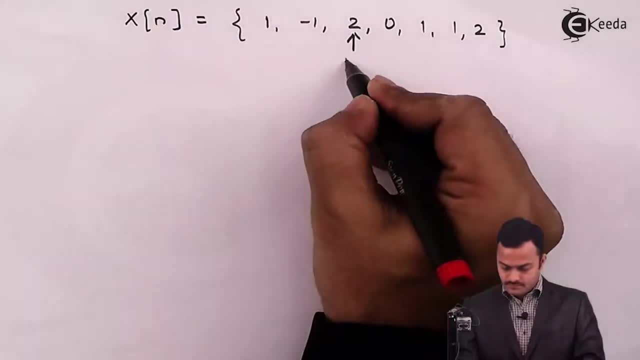 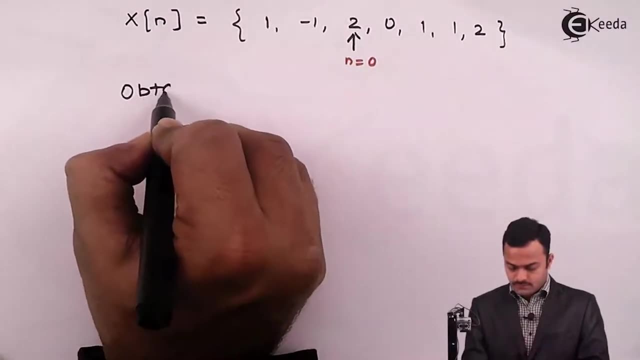 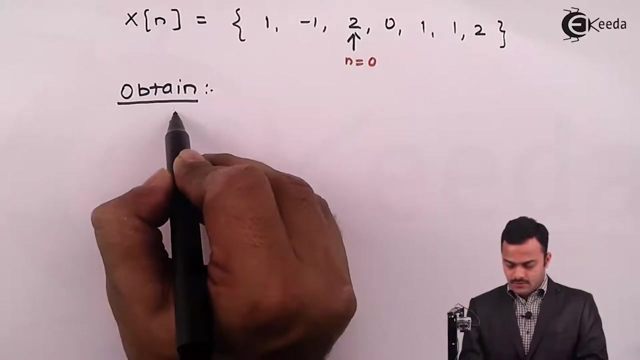 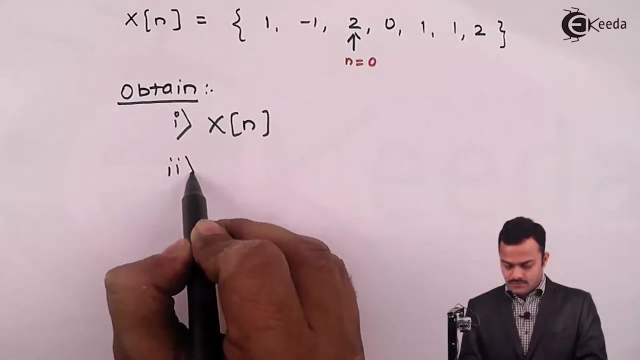 This is n equal to 0 point, And for this signal we have to obtain, Obtain means, we have to plot all this. First, a signal itself X of n, Then second, X of minus n. Third, we are having X of n minus 2.. 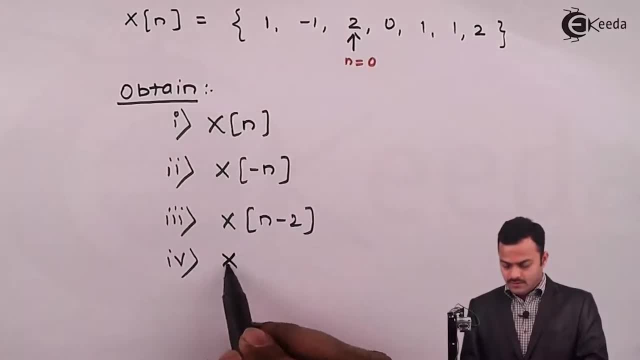 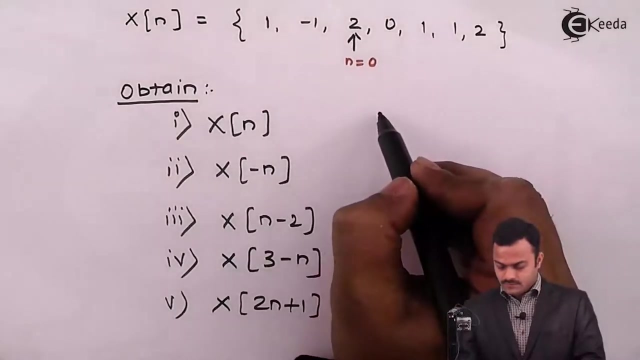 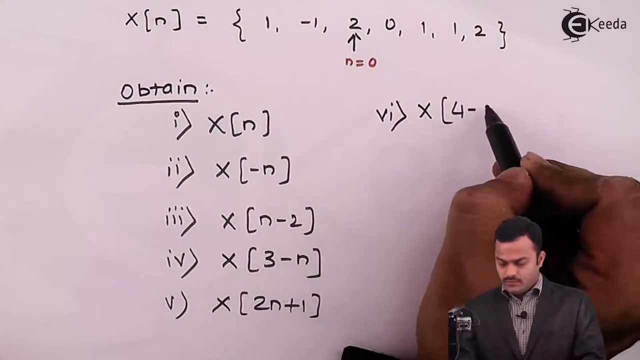 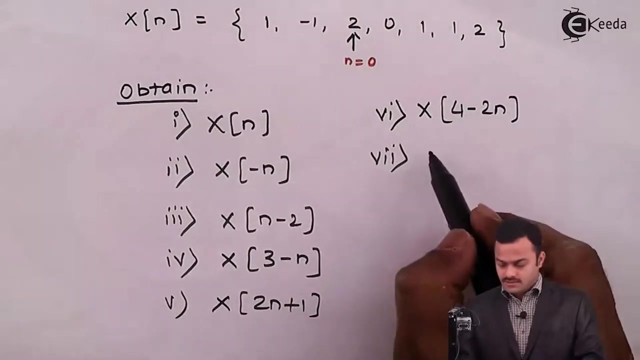 Okay, Then we are having X of 3 minus n. Next we are having X of 2n plus 1.. Next, X of 4 minus 2n. Next, X of 4 minus 2n. Okay, 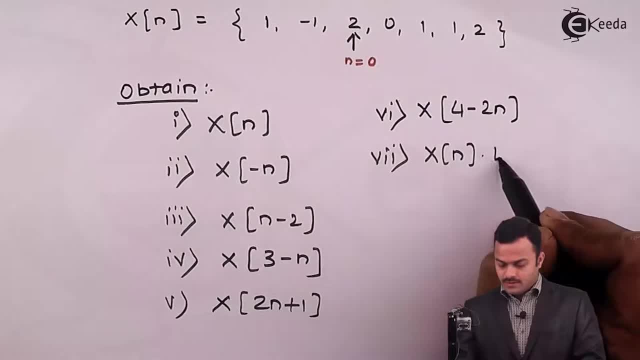 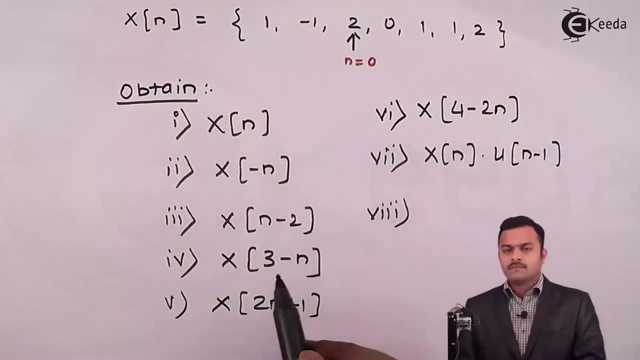 x of n multiplied by u of n minus 1, then x of n minus 1 multiplied by delta, n minus 2, so on. So what we have done over here, one problem we have taken of a discrete time sequence and almost all the properties we have covered over here. So let us solve this. 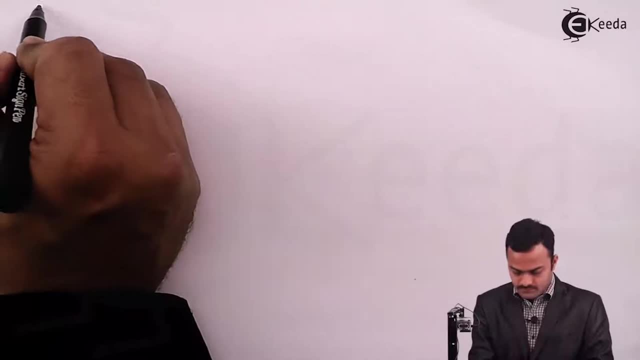 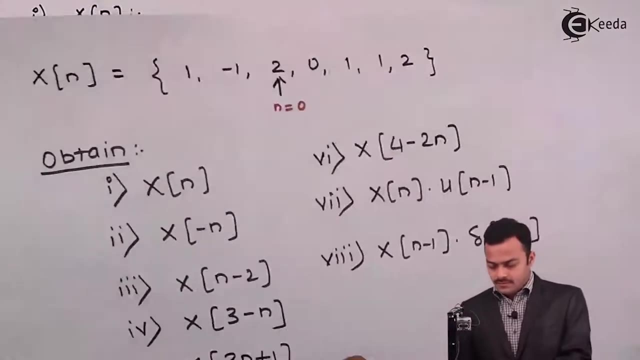 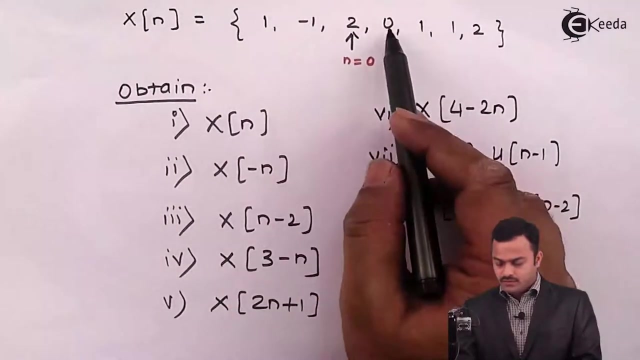 First is to obtain x of n. It is quite simple: Over here, on our n axis this is n equal to 0, rest it can be a minus 1, minus 2. over here, 1, 2,, 3,, 4,, 5,, 6,, 7,, 8,, 9,, 10,, 11,, 12,. 12,, 13,, 14,, 15,, 16,, 17,, 18,, 19,, 20,, 21,, 22,, 23,, 23,, 24,, 25,, 26,, 27,, 28,, 29,, 30,, 31,, 31,, 32,. 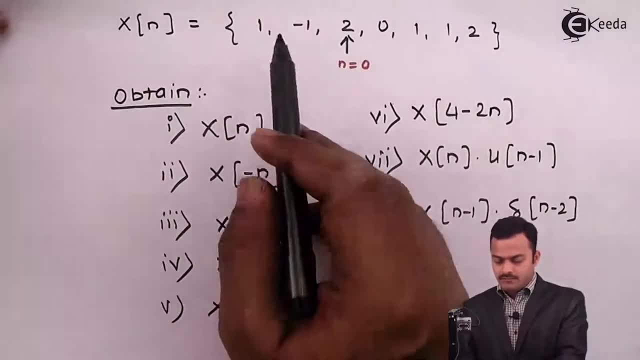 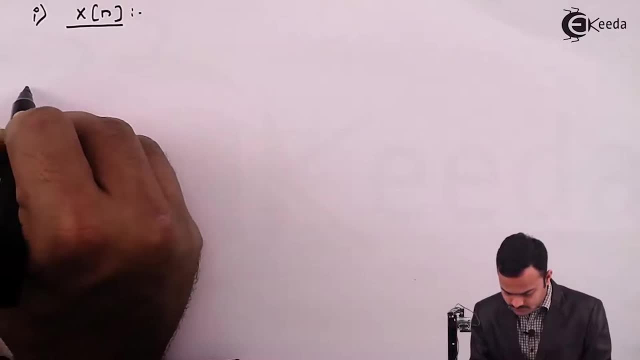 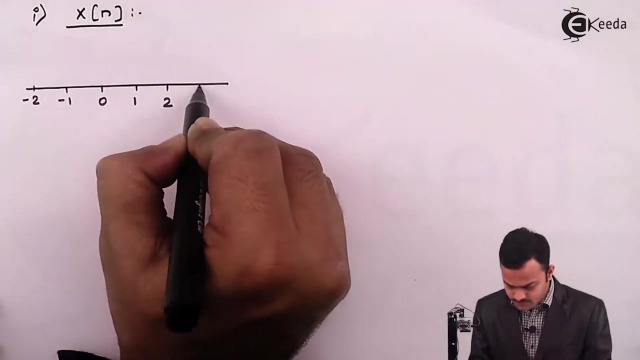 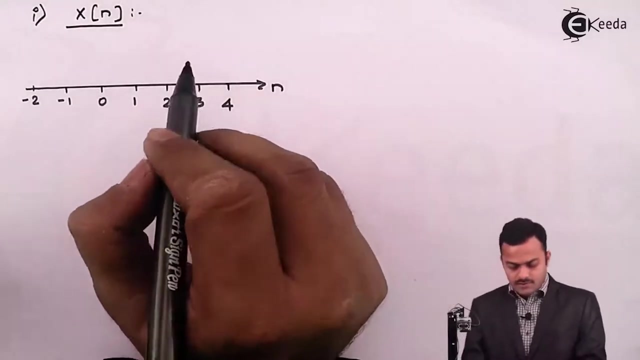 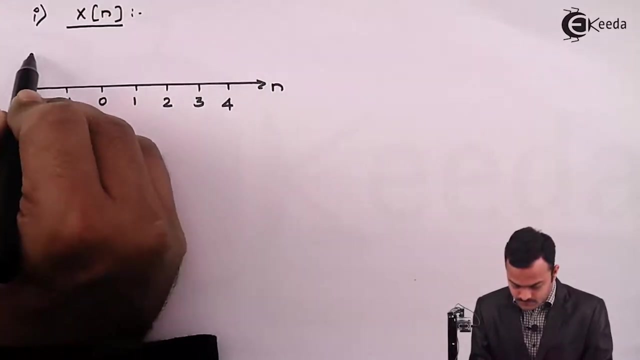 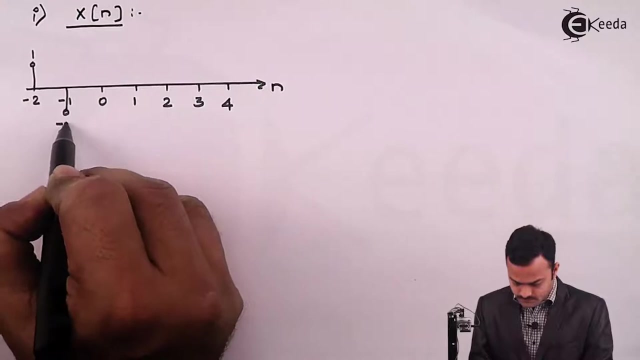 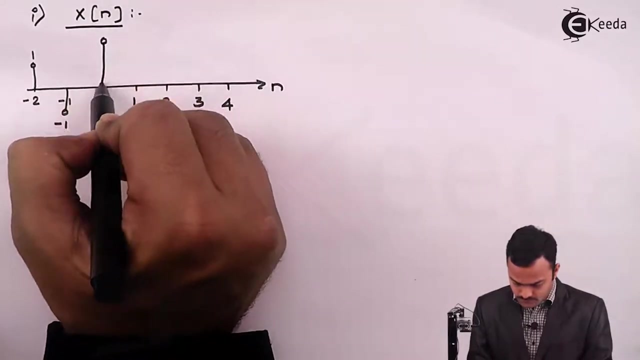 34.. So the signal span will be from minus 2 to 4.. So for n equal to minus 2, it is having a value 1.. For n equal to minus 1, it is minus 1.. For n equal to 0, it is 2.. For n equal to 1, it is 0.. For n equal to 1, it is 0.. For. 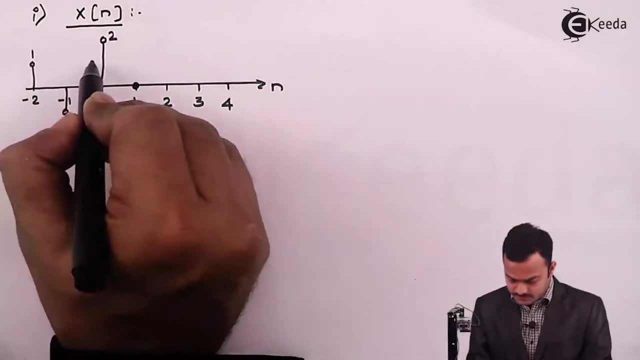 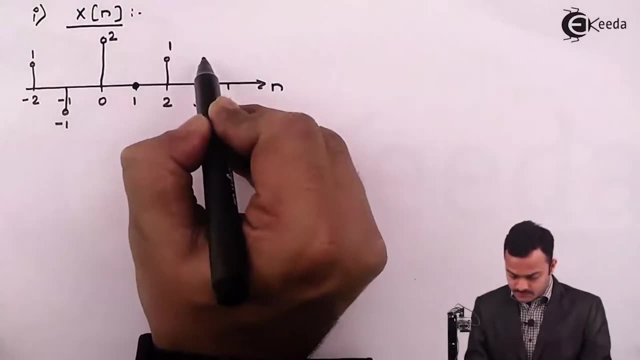 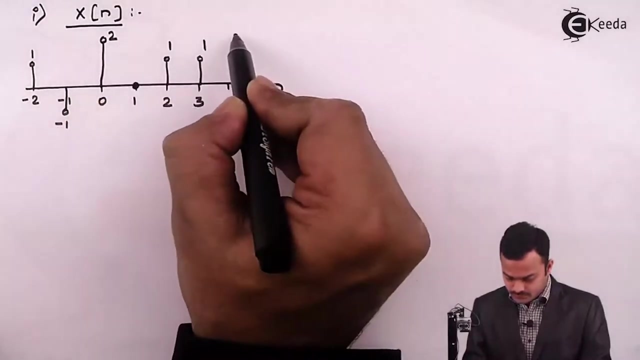 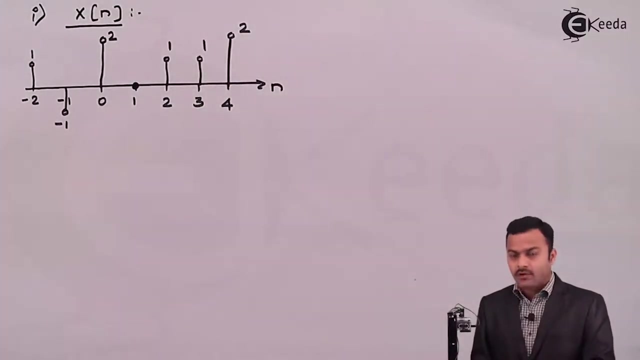 n equal to 2, it is 1.. For n equal to 3, it is once again 1.. And for n equal to 4, it is 2.. So this is x of n, Quite simple. Next, we want: x of n is equal to minus 1.. So this: 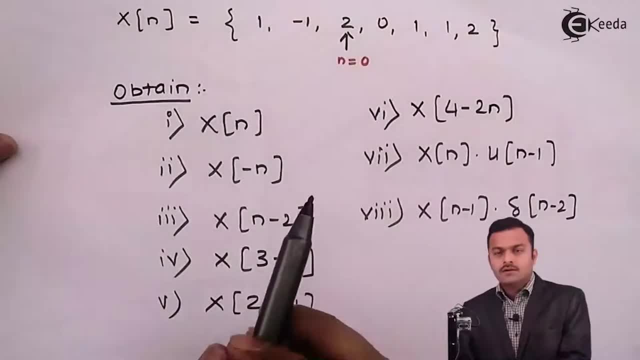 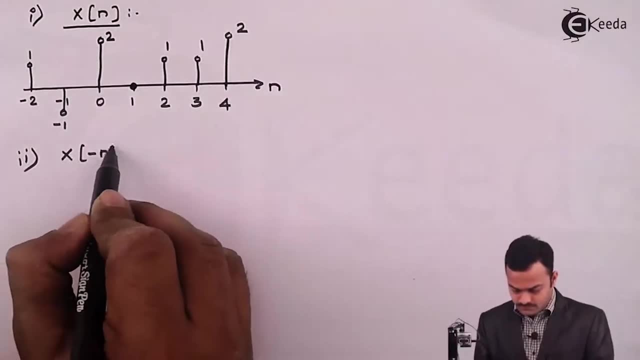 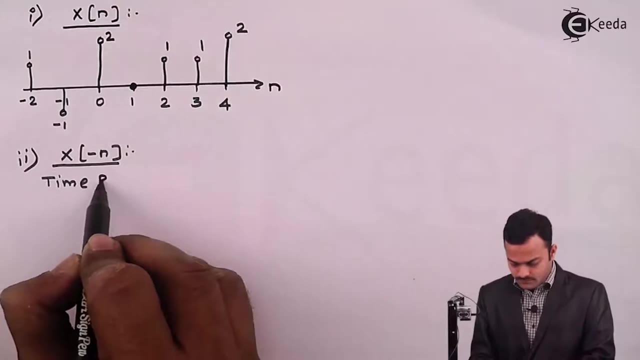 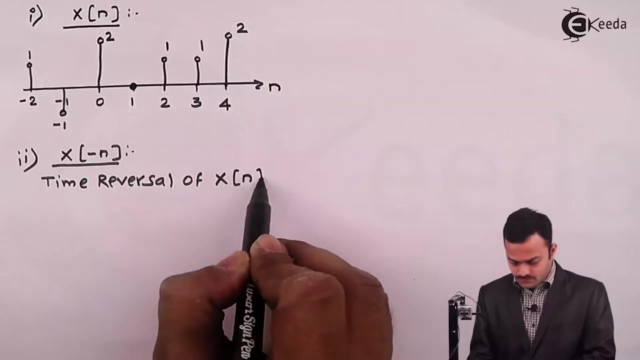 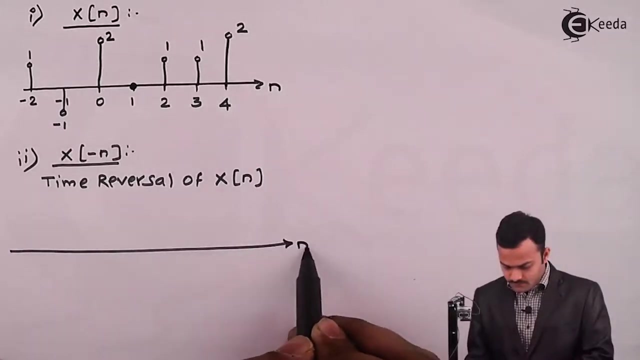 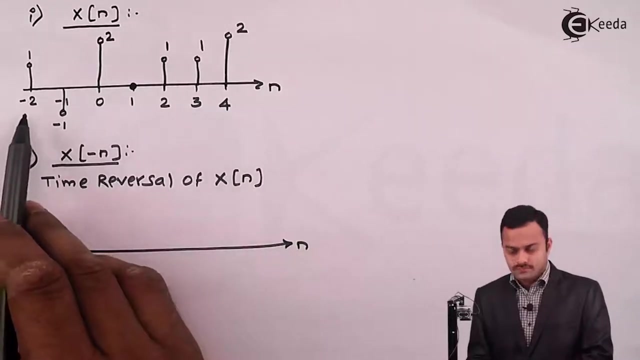 is x of minus n. So we need to do a time reversal of x of n. So how the signal will be obtained: This time signal will have the span from minus 4 to 2.. So something like this we will. 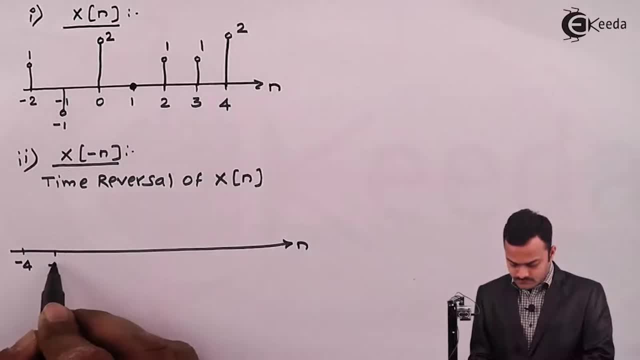 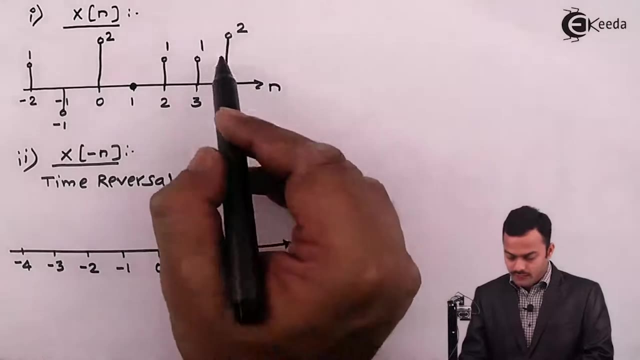 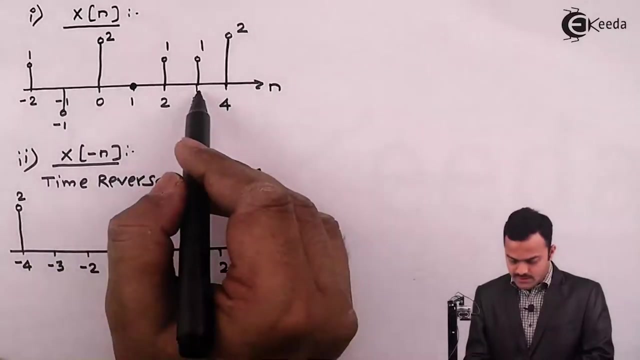 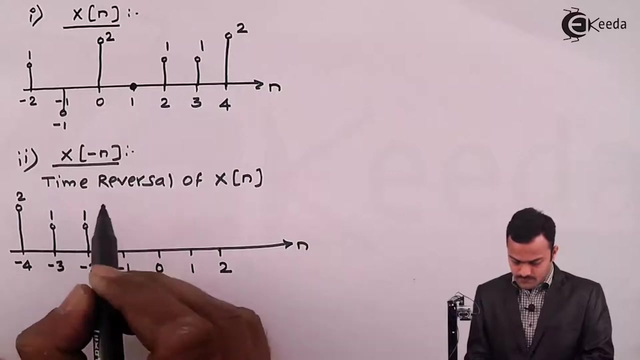 get. So. for minus 4, we will have value 2.. Minus 3, it is 1.. Minus 2, it is 1. once again, For minus 1, it will be 0.. For 0, it will be. 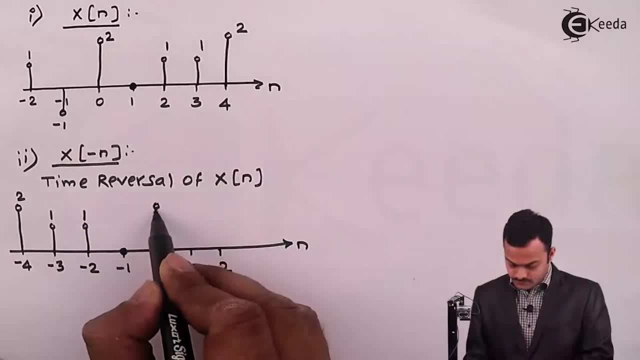 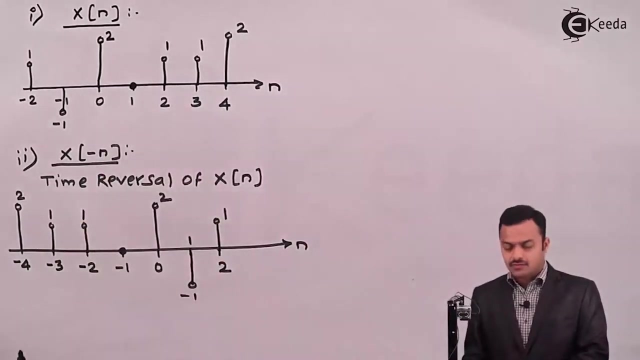 2.. For 1, it will be minus 1.. So this is instant 1.. And for 2, it is 1.. So just a time reversal of original signal will give you x of minus n. Let's go ahead for the third. 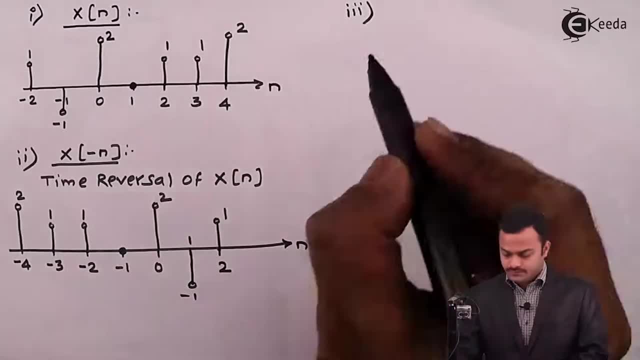 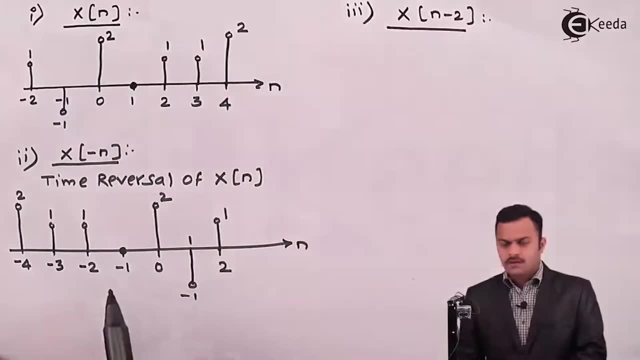 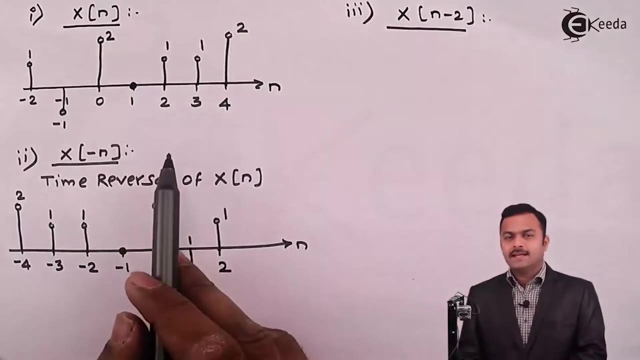 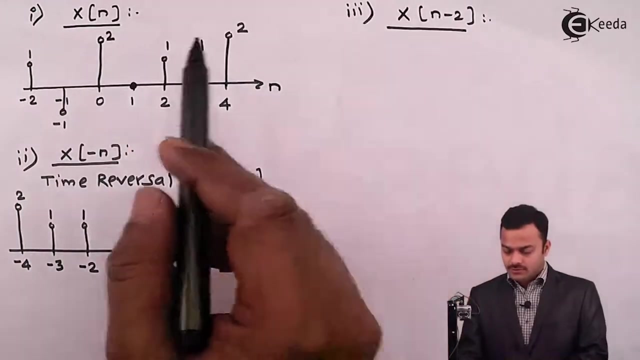 So third signal is x of n minus 2.. This is x of n. How to get x n minus 2?? Minus 2 means this is a delay. delay by 2 unit Delay means it is away from the y-axis towards right. So I need to delay, shift this signal. 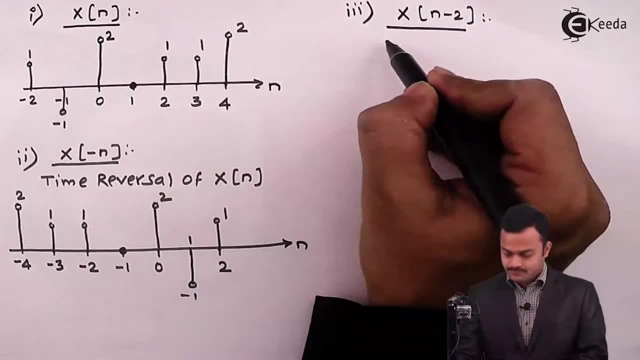 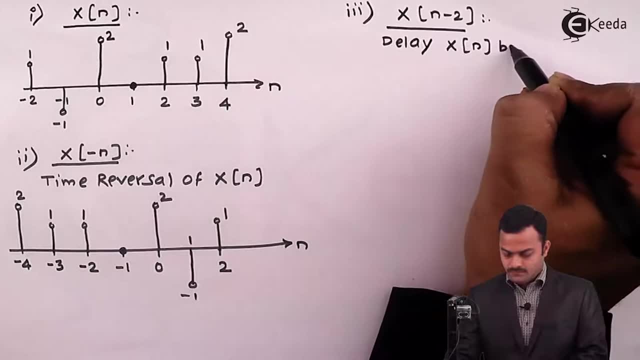 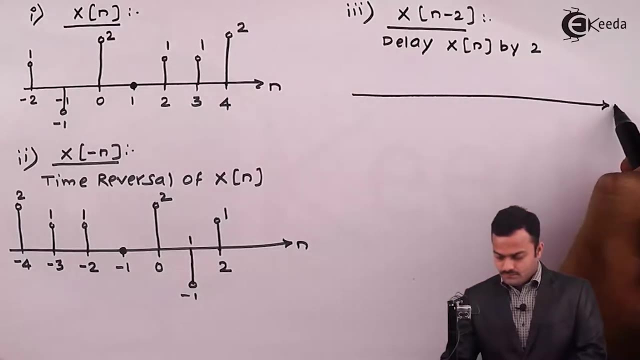 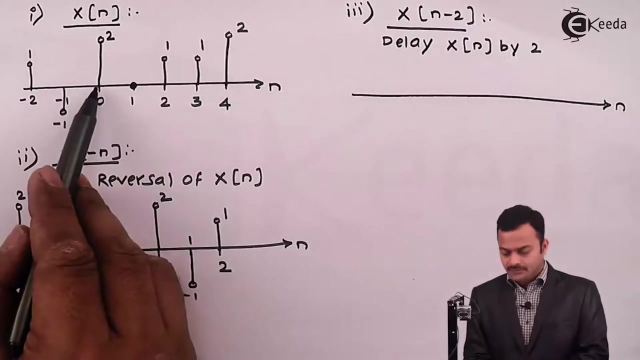 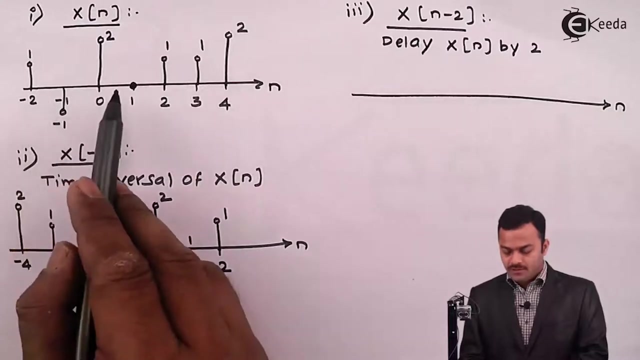 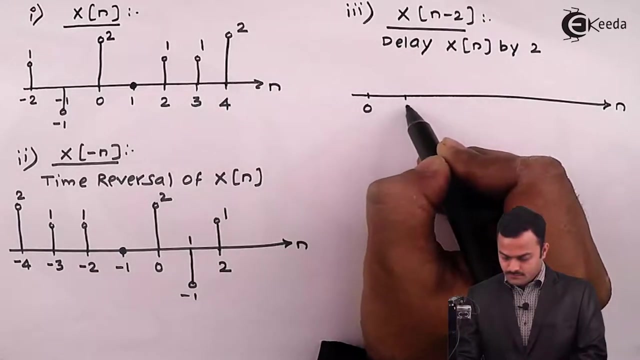 by 2 unit to the right side. So if I delay it by 2 units, obviously this minus 2 will get shifted to 0 and this 4 will get shifted to 6.. Basically we will have the span of the signal from 0 to 6.. 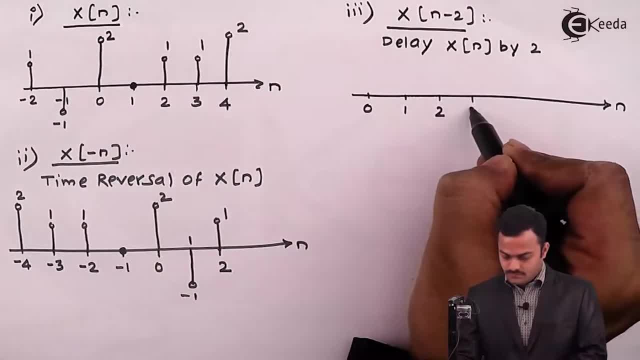 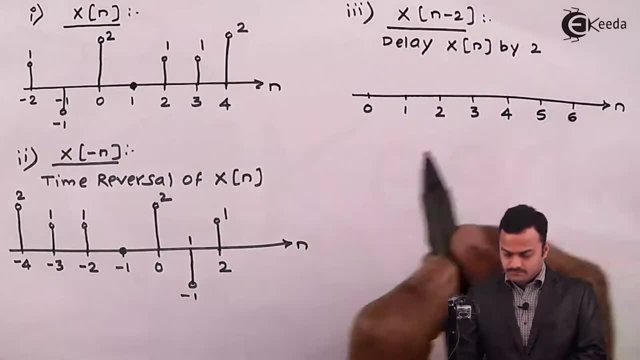 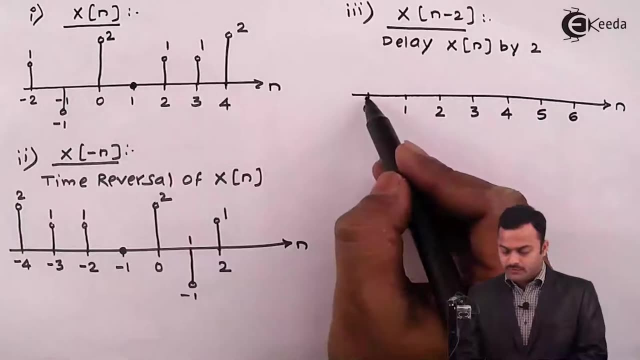 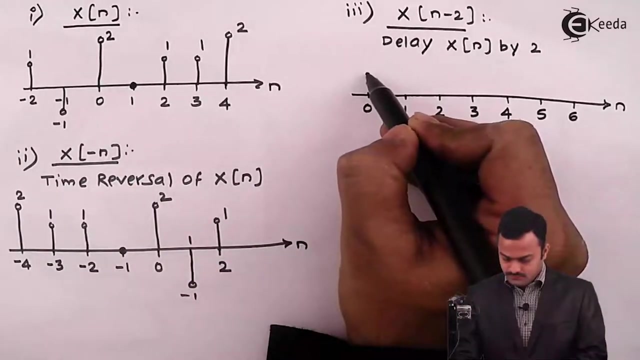 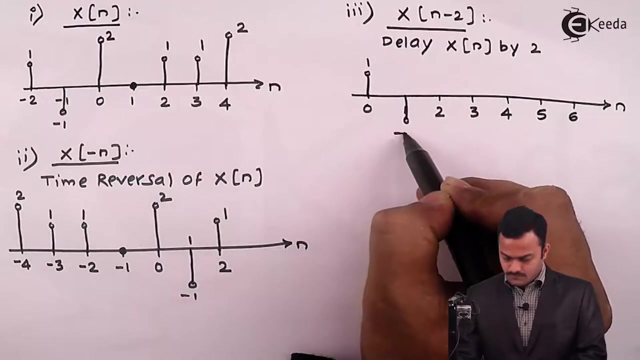 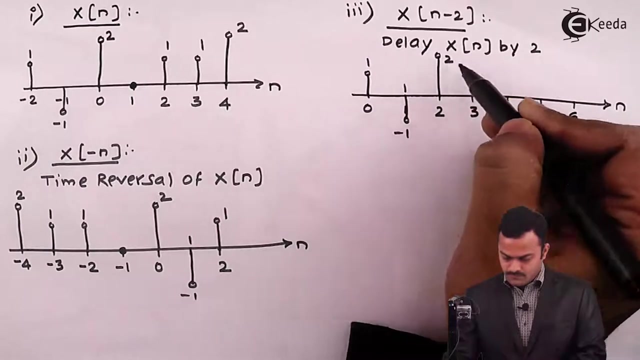 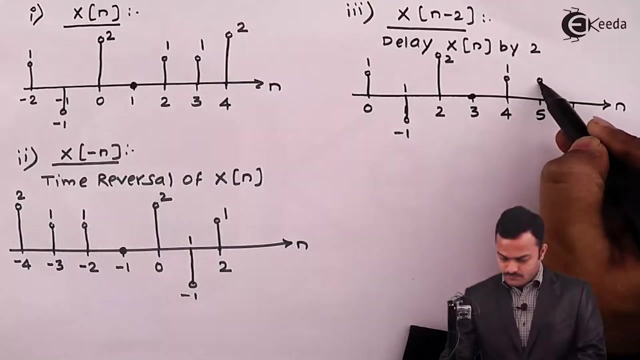 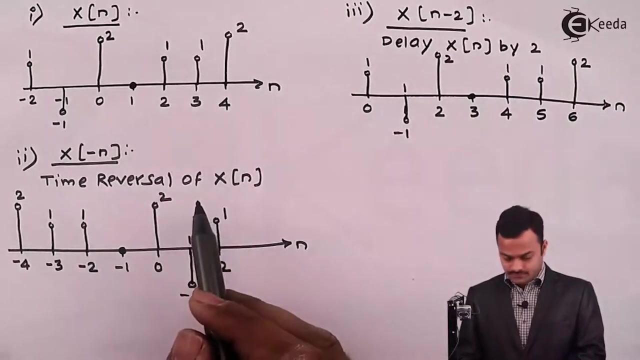 So whatever the value for n equal to minus 2 in case of x of n, that will be the same over here for 0 and likewise. So we will get a signal like this: So this is a time delayed version of x of n. Let us go ahead. Fourth signal that we 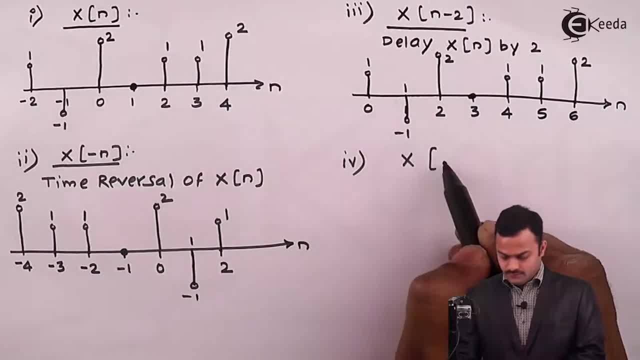 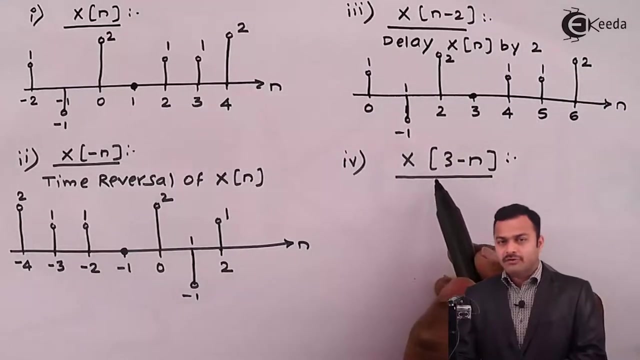 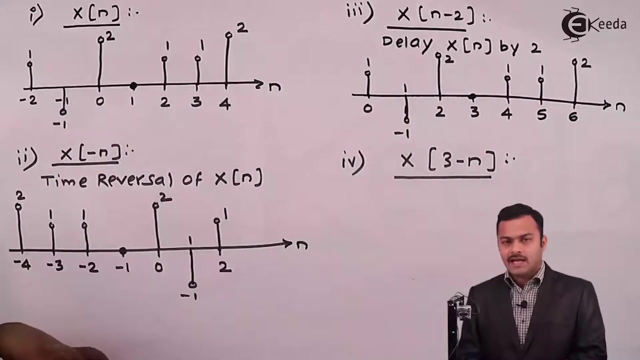 need to obtain is x of 3 minus n. So over here two operations are obtained. One is time advance and second is time reversal. So first, as per the priority, we need to do a time shifting. So plus 3 is the shift. That means advance x of n by 3 units. 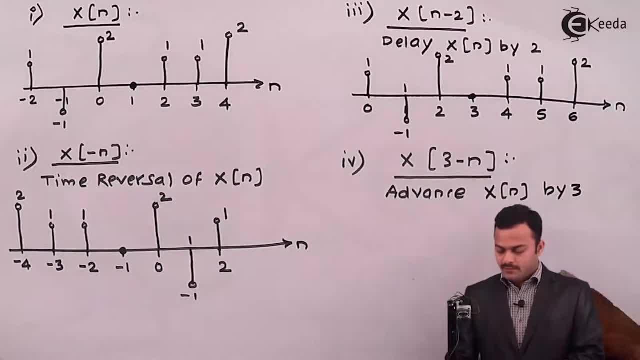 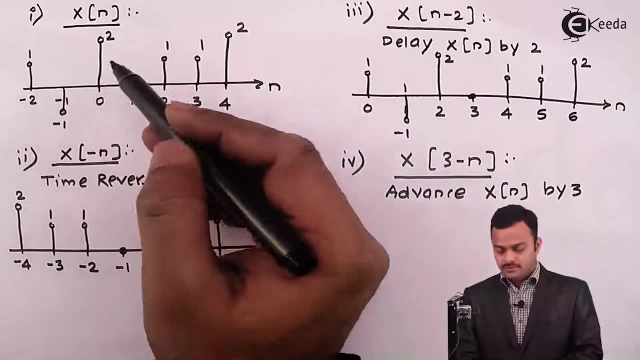 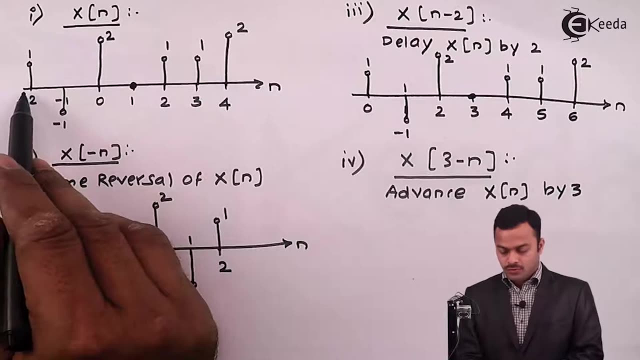 So the signal that we obtain will be x of n plus 3.. So this: I need to shift to the left, towards y axis, by 3 units, So the span will be from minus 5 to 1.. Let us see how. 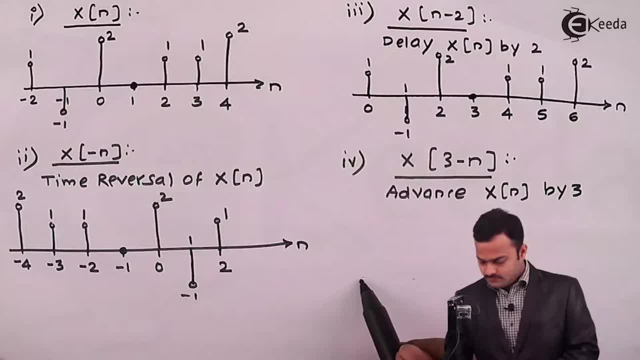 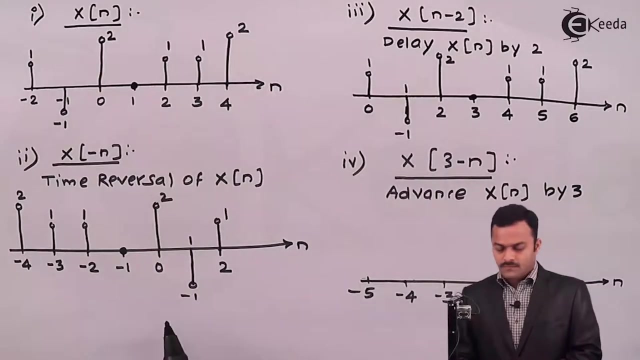 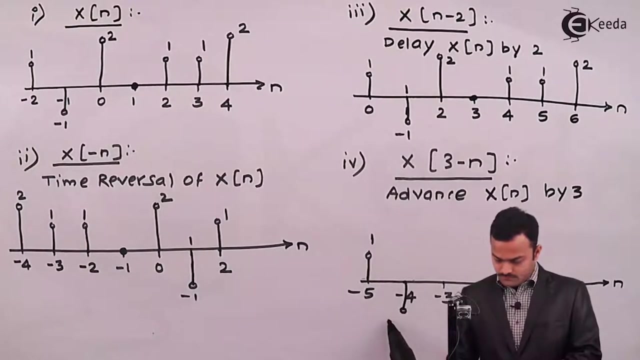 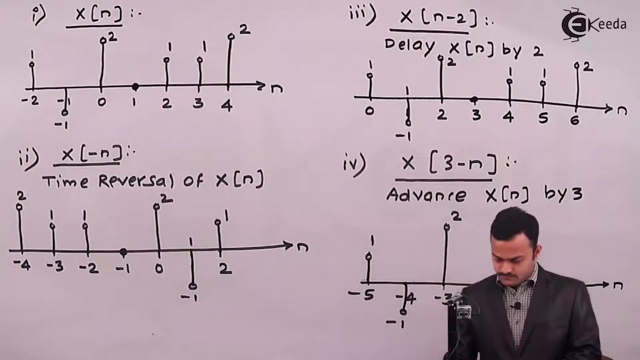 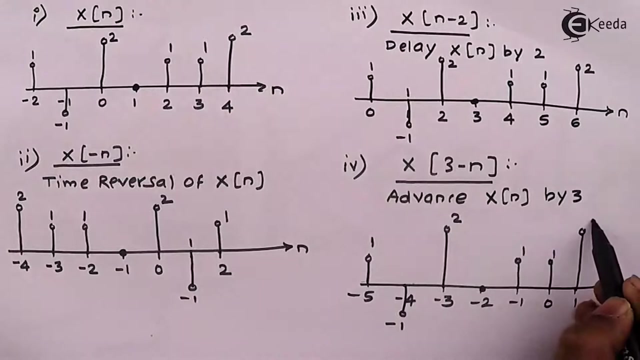 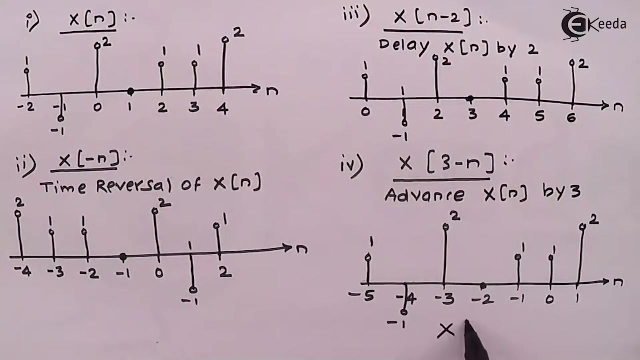 the signal will look like: So for n equal to minus 5, I will get a signal equal to 1.. So over here I obtain a signal which is the advance version of x of n, That is, nothing but x of n plus 3.. 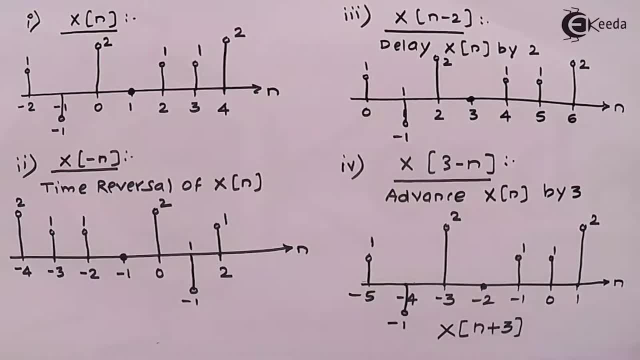 So over here I obtain a signal which is the advance version of x of n. That is nothing but x of 3.. But what we want is x of 3 minus n, So n need to be replaced by minus n, and 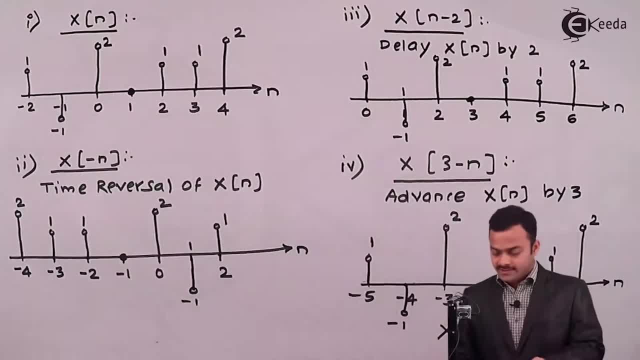 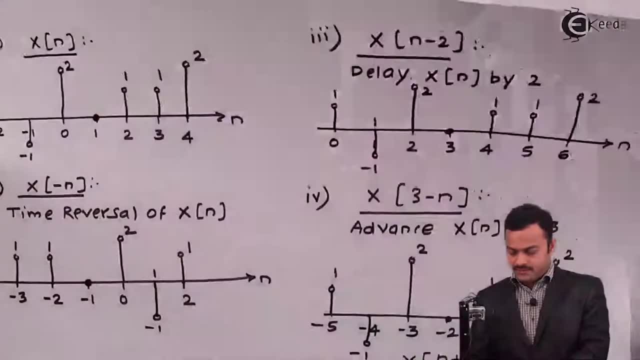 that is nothing but a time reversal of this signal. So next step, we will do a time reversal of x of n plus 3.. So let us do time reversal of x of n plus 3, which will give x of 3 minus. 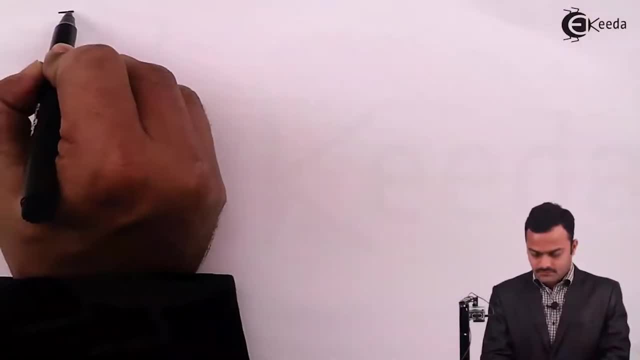 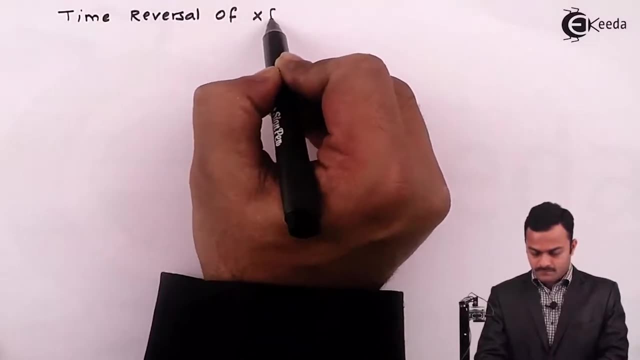 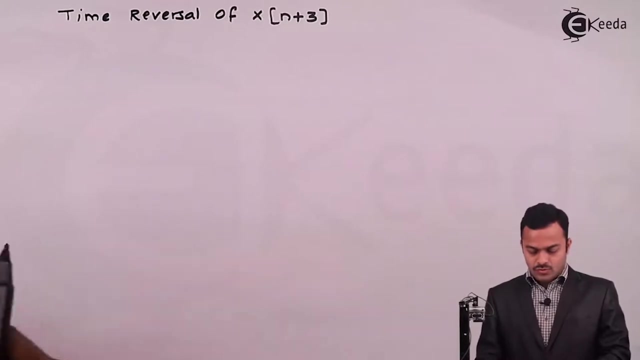 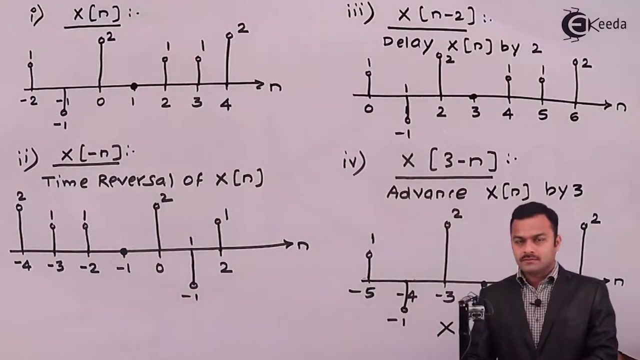 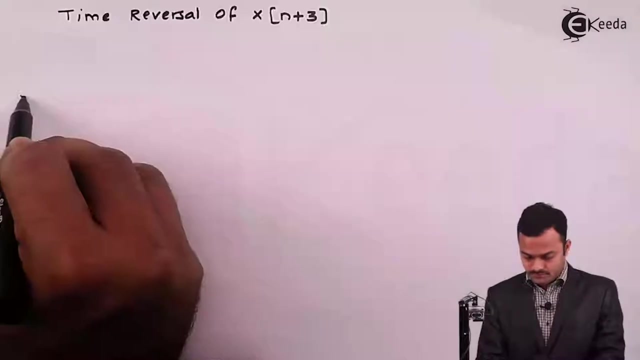 n. Let us see how That means. n axis will be replaced by minus n. So whatever values we got in, y axis will get reverse Meaning span of the signal now will be from minus 1 to 5.. So this is the time reversal of x of n plus 3.. So let us do time. reversal of x of n plus. 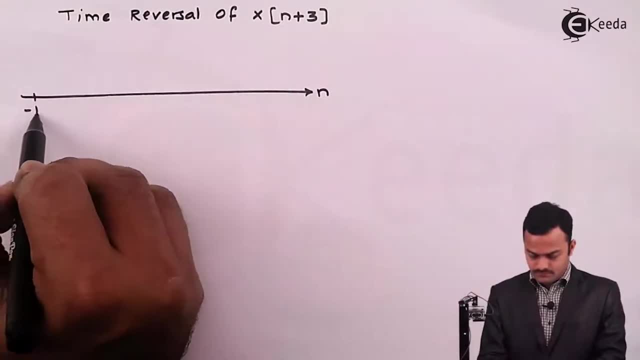 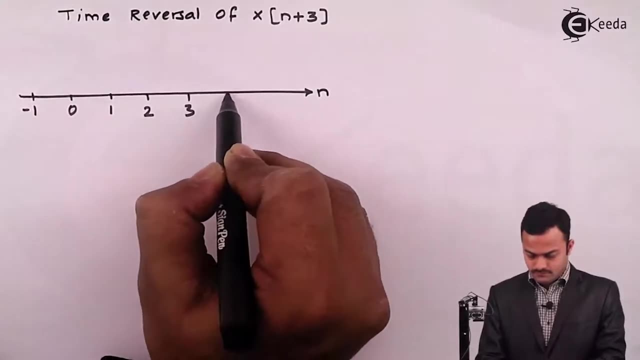 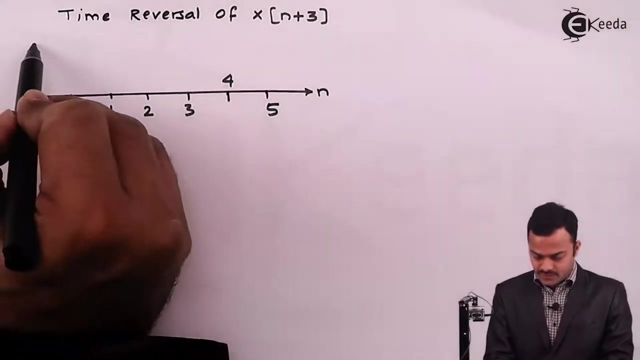 3.. So we will get a signal like this: For n equal to minus 1,, it is 2.. And for 0,, it is 1, and likewise. So we will get a signal like this: For n equal to minus 1,, it is 2.. And for 0,, it is 1, and likewise. 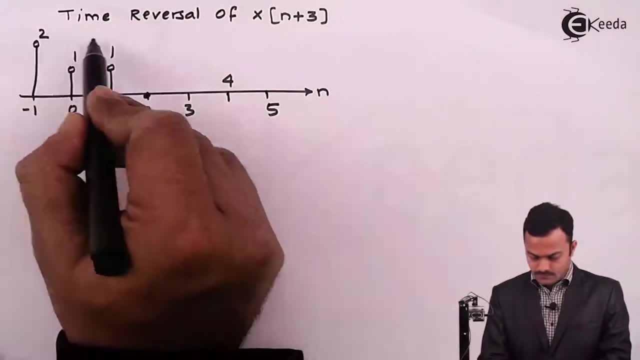 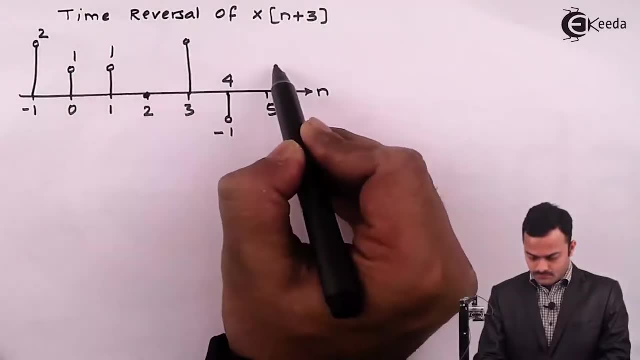 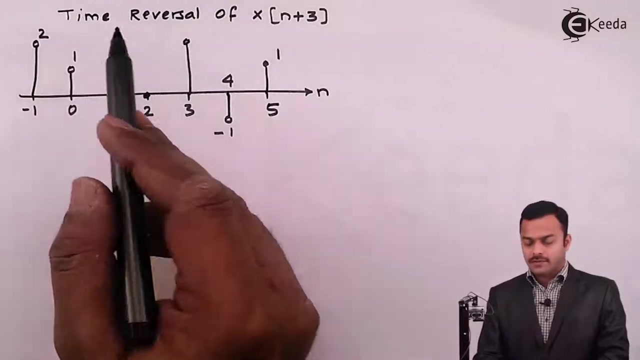 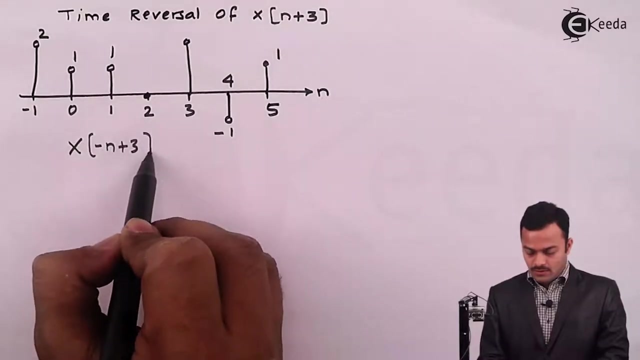 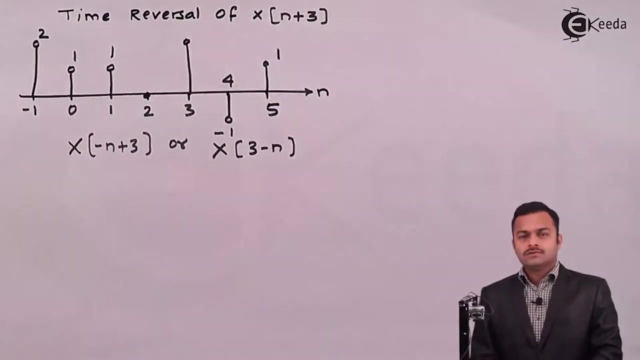 So this signal that we obtained is doing time reversal of x of n plus 3, which is nothing but x of minus n plus 3, or I can write this as x of 3 minus n. So that was 4th signal. Let us go to the next. 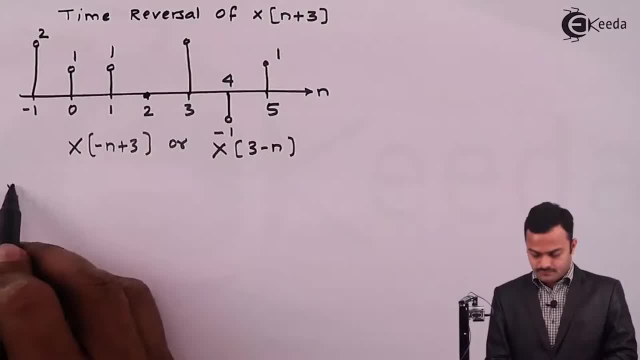 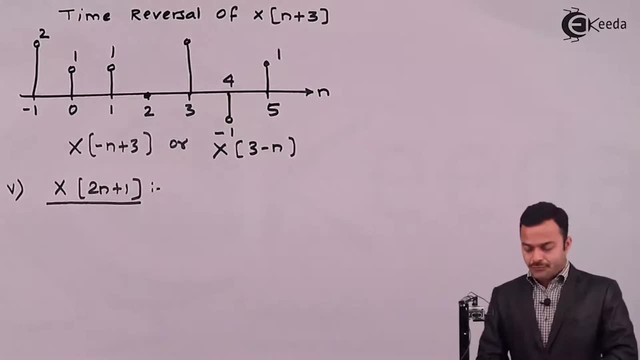 5th one. In 5th one we are supposed to get, we are supposed to get x of 2n plus 1.. Now, to get x of 2n plus 1, we need to take a help of x of n and, as per the priority, first. 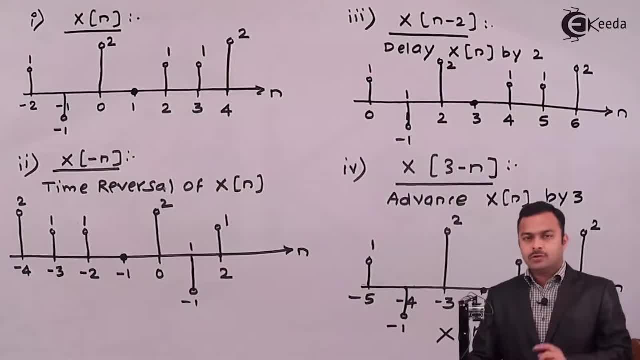 we will shift this x of n and then we will do the time scaling. Then, if you want, you can shift it like this: Now they are your giving these seven times twelve zeros for n, but they have five times n. No, we cannot等 this n, Not before you know that and get driven by a point så amazing. 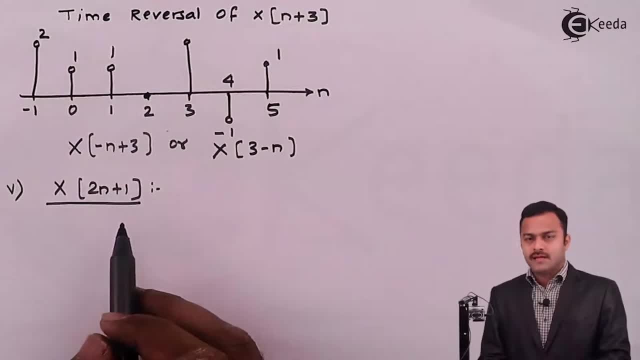 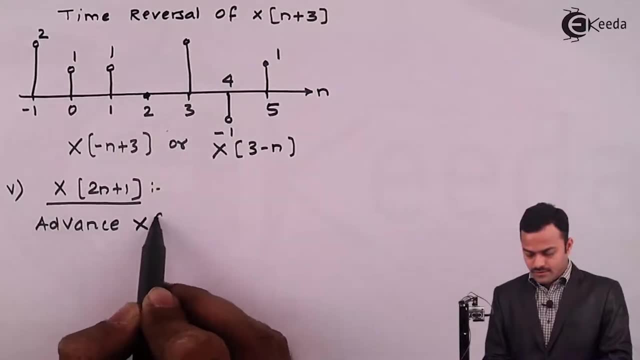 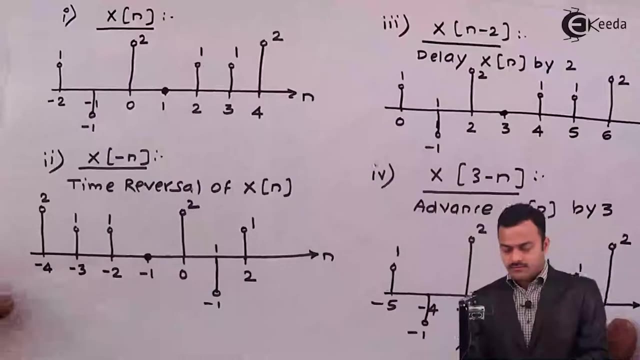 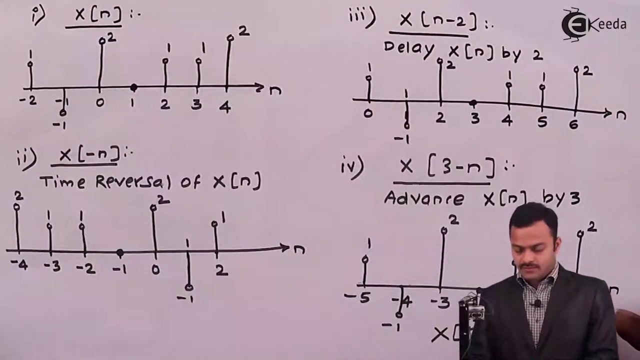 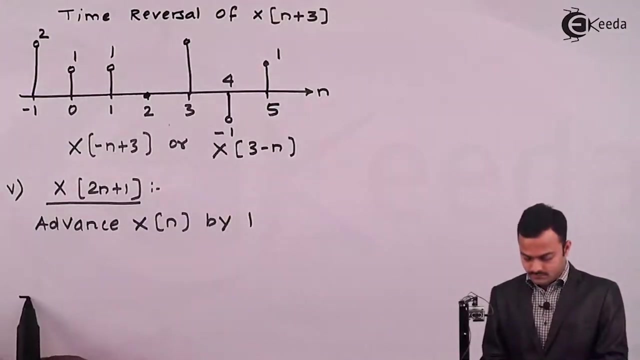 so plus one is the shift, plus means advance. so let's advance x of n by one unit. advance means it is towards y axis in negative n side. so the span of the signal will be from minus 3 to 3. so so signal will be like this: 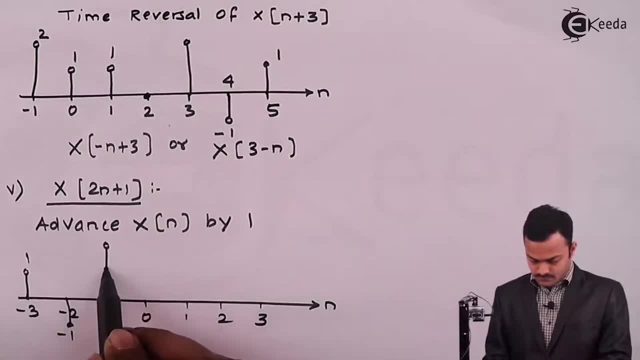 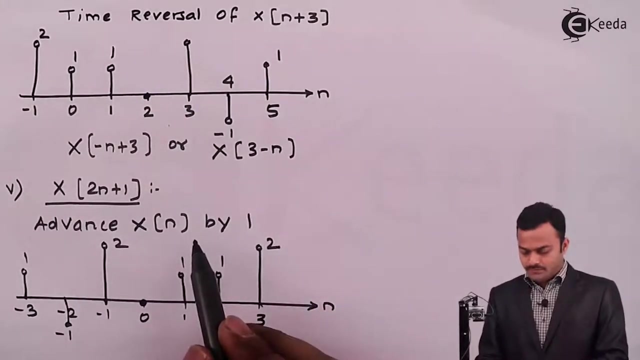 so. so after advancing x of n by one unit, the signal we obtain is x of n plus one. but what we want x of 2n plus 1. so n is getting multiplied with the 2. that mean it is a compression. so we have to compress this signal by 2 unit. 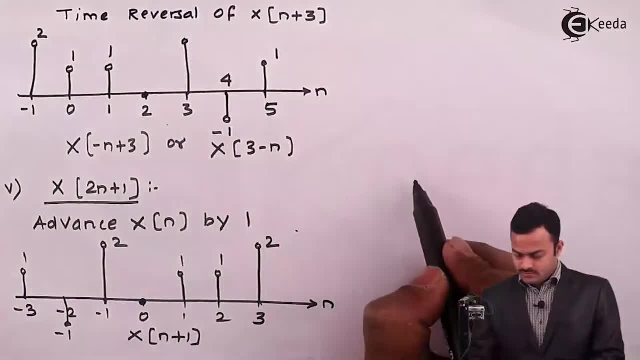 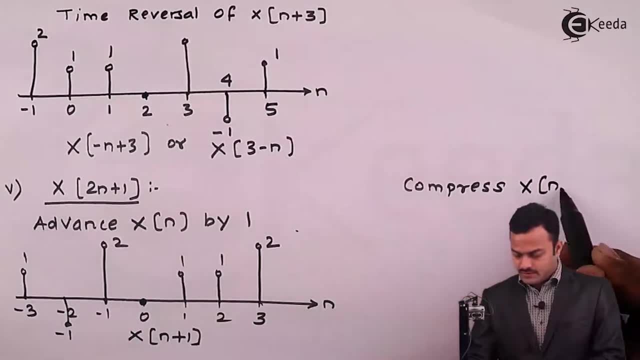 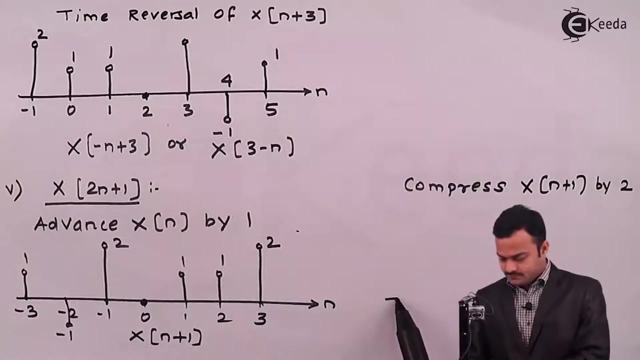 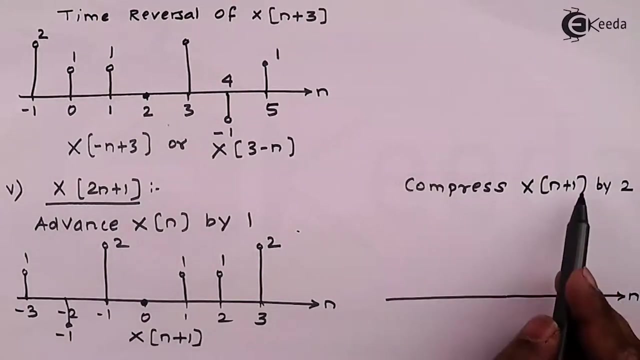 so we are doing this over here. so we will compress x of n plus 1 by 2.. now we need to be careful, because whenever discrete time is compressed, there is a possibility of losing some of the data. now, this need to be compressed. so, as for the logic, all the n points we need to divide by 2. 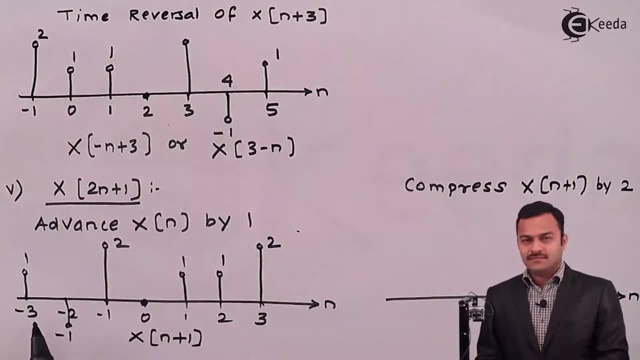 so minus 3 by 2, but that is not an integer. hence the problem is that this data is going to be lost. same will be the case for this minus 1, because if i divide by 2, it will become minus 1 by 2, which is not an integer. so unfortunately, this will also be lost. 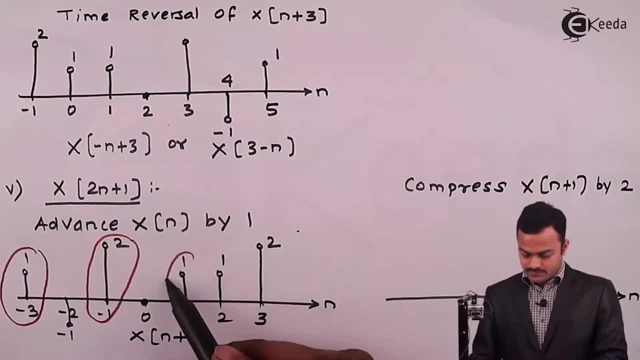 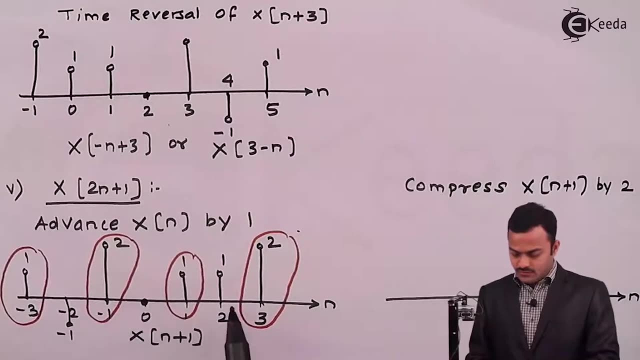 same thing will happen for n equal to 1 and n equal to 3, so these data points are going to be lost. so what is left is just this minus 1, this 0 and this 1, and that exists at n equal to minus 1, 0 and 1.. so in the end, the signal that we obtain will be like: 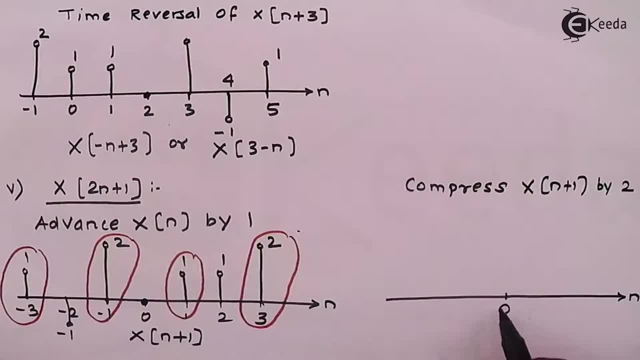 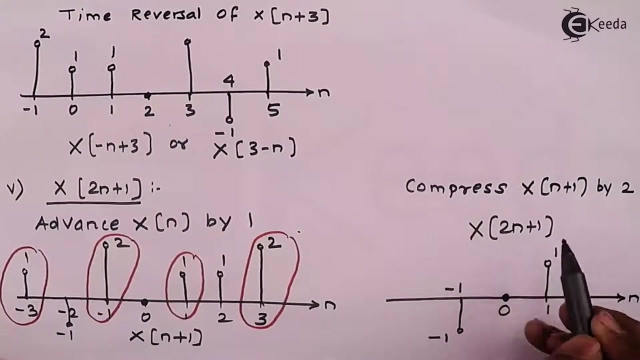 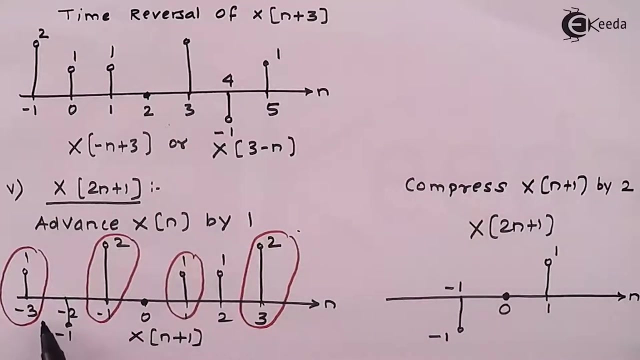 this: for minus 1, we will get a value minus 1 only. for 0 it is 0 and for 1 it is 1. so this is x of 2n plus 1. whenever we compress a discrete time sequence, it is the possibility that some of the data points will be lost. 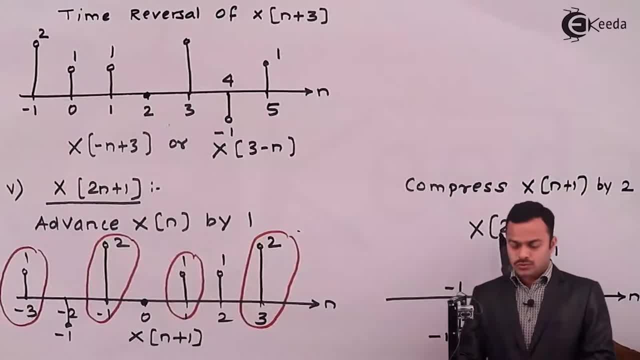 data points will be lost which are not multiple of 2.. so 3 1 minus 3 minus 1 in this case were not the multiples of 2, hence data points corresponding to those particular values of n will be lost. let's go to the next signal. 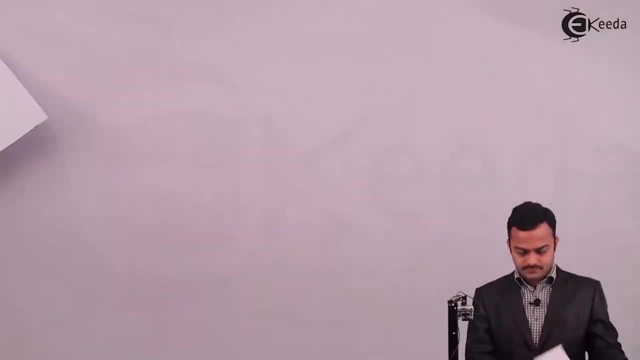 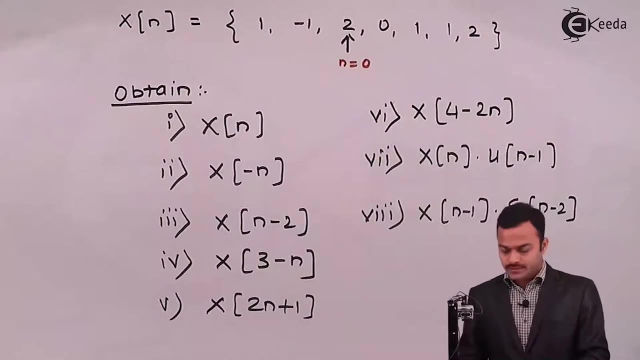 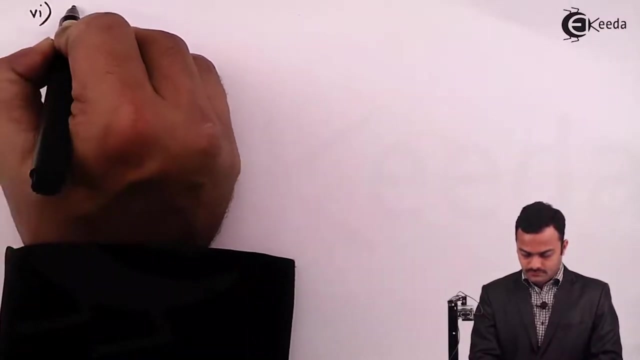 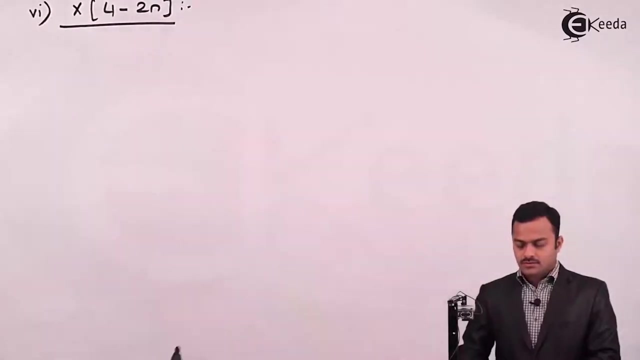 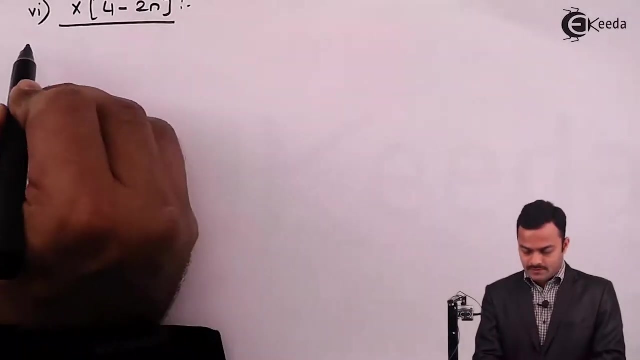 So sixth signal over here is x of 4 minus 2n. So here three operations are need to be performed: One is a shifting, second is a scaling and third is the time reversal. So the priority is always given to shifting. 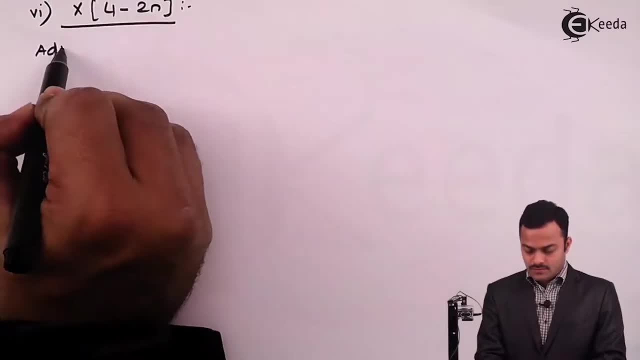 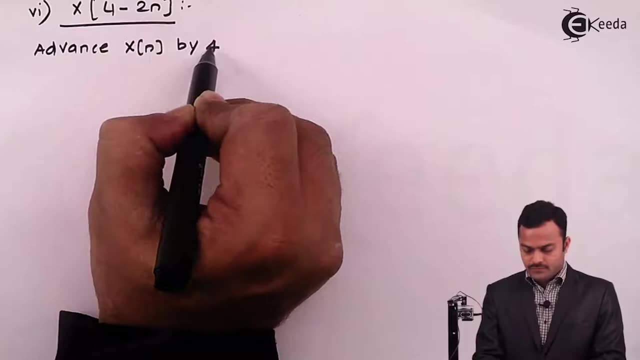 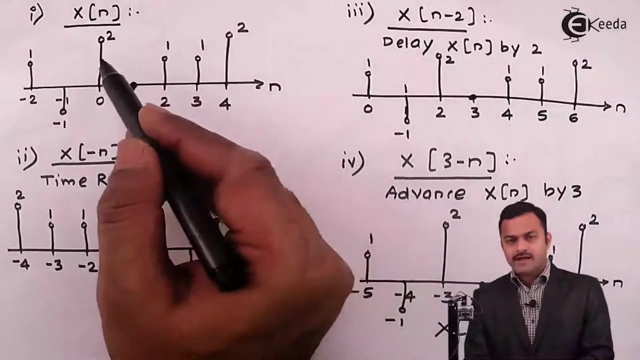 So we will advance because there is a plus 4.. So advance x of n by 4.. So x of n is like this: we need to advance it, that mean towards y axis in the left hand side direction, By 4 unit. 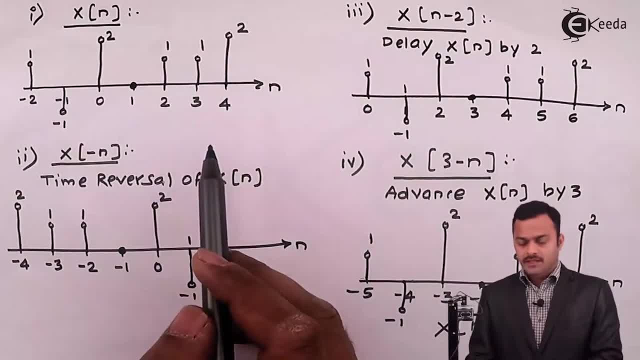 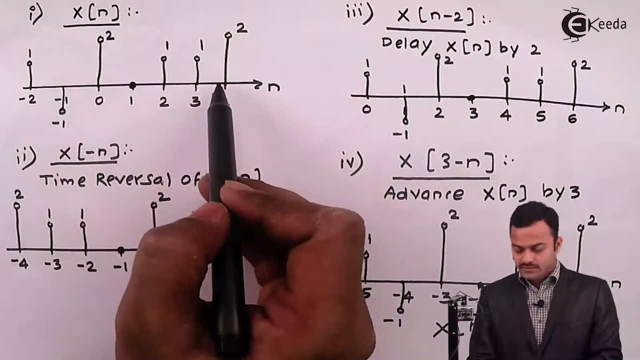 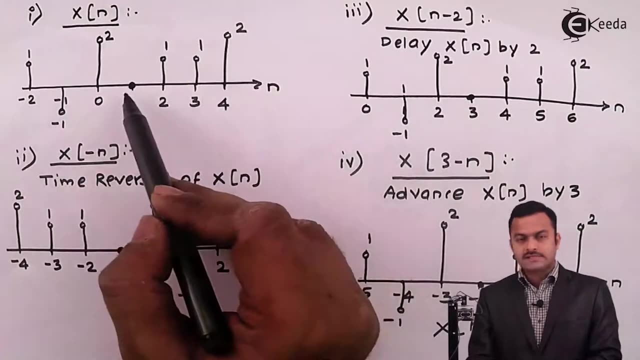 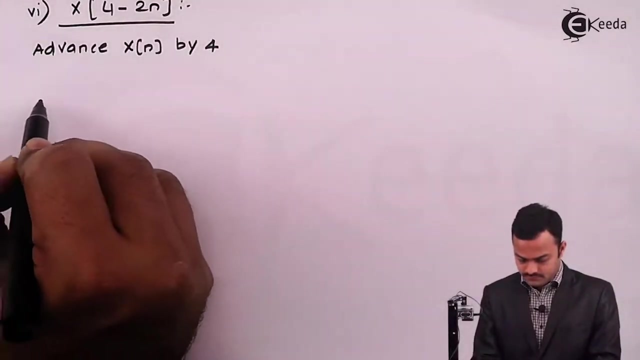 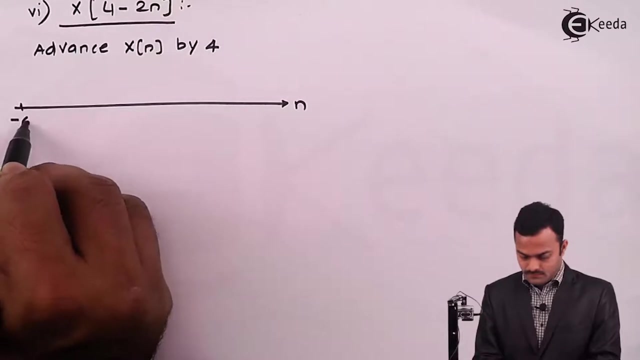 So span of the signal will be minus 6 to 0 because we need to shift this side by 4 units. So 4 units over here get shifted, So minus 6, and over here it is 0.. 1. 2. 3., 4., 5., 6., 7., 8., 9., 10., 11., 2., 1., 2., 3., 4., 7., 2., 8.. 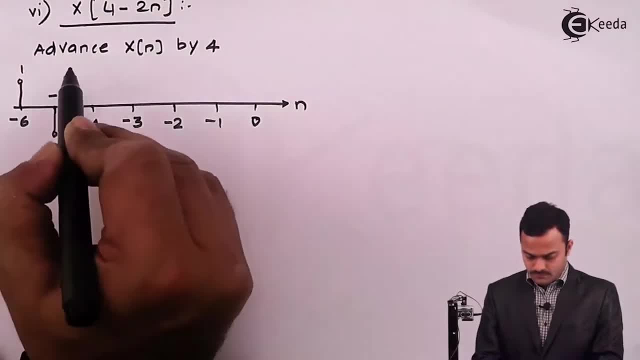 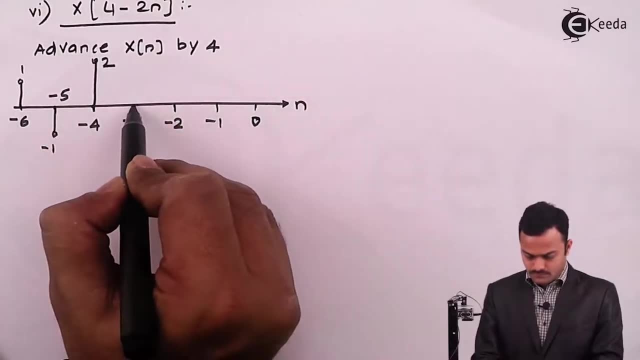 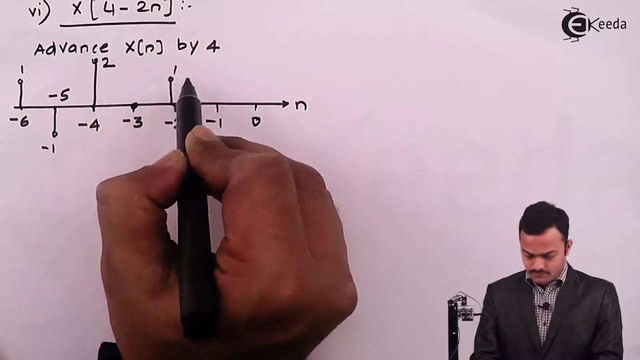 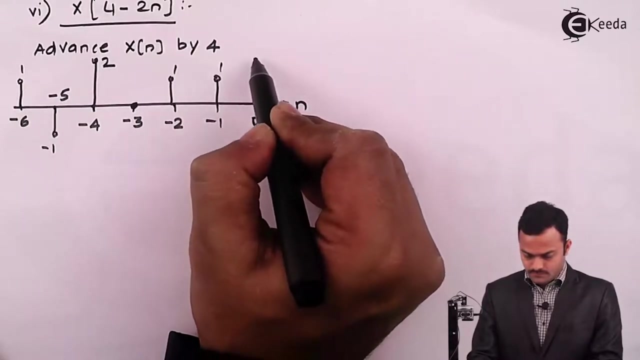 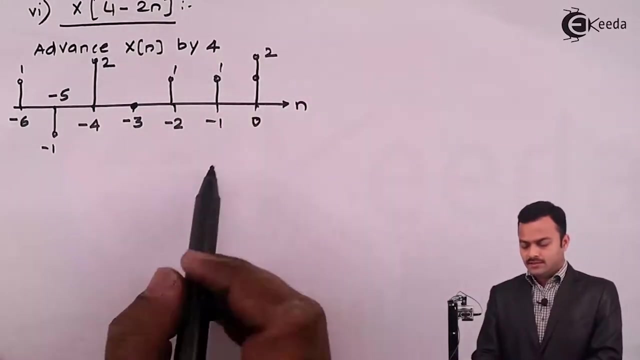 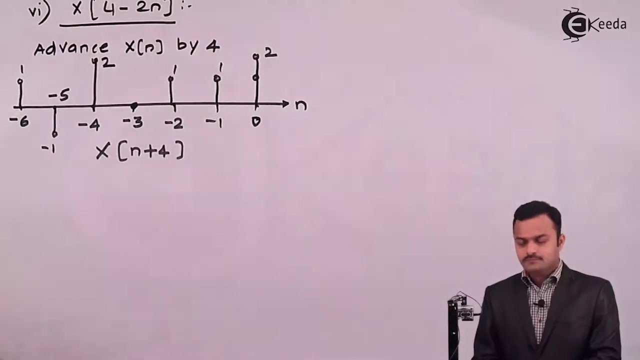 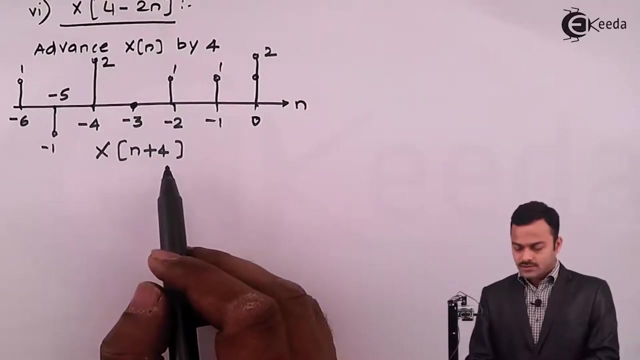 9. 1. 2.. So we will get a signal which is shifted to left side by 4 unit. This is x of n plus 4.. Next, either we can do a time reversal or time scaling. So first just do a time scaling. So it is 2n, So need to be multiplied by 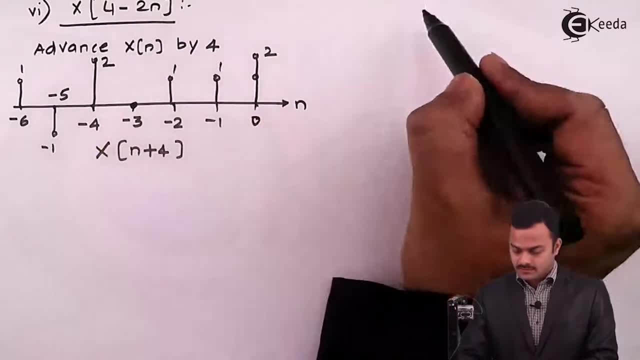 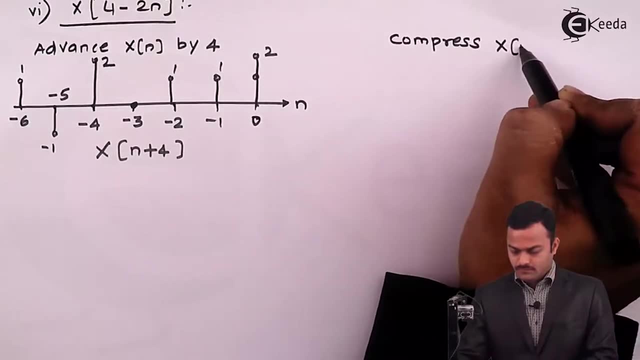 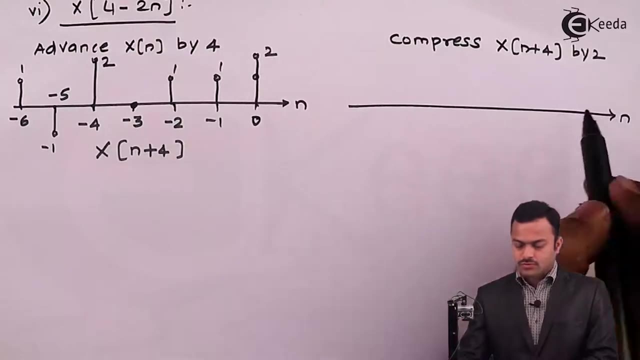 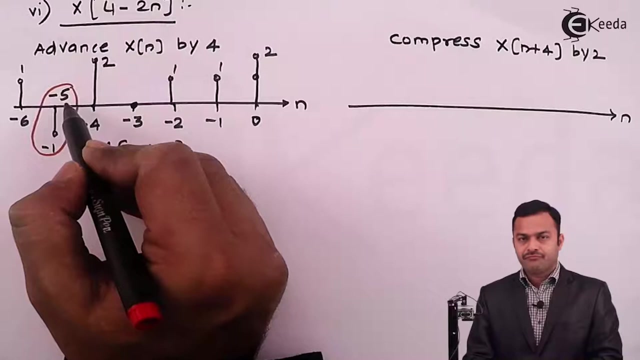 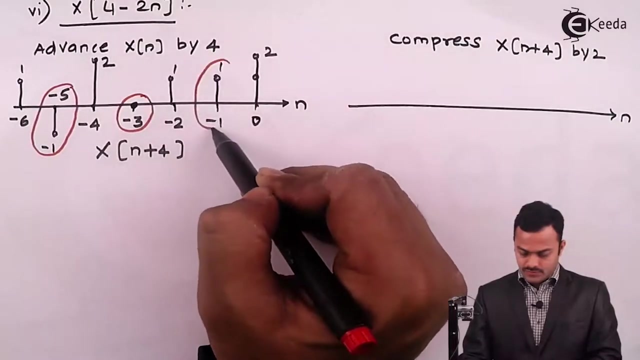 2 means it is a compression. So compression sum of the data will be loss and the data which is not multiple of 2 will be loss. So here there will be some loss points. This point will get loss because minus 5 is not a multiple of 2.. This point will get loss. Similarly, this point will also. 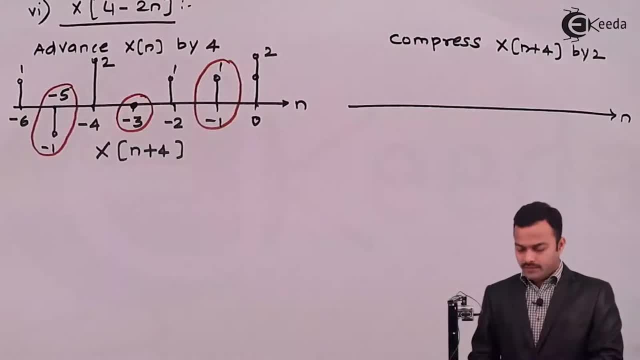 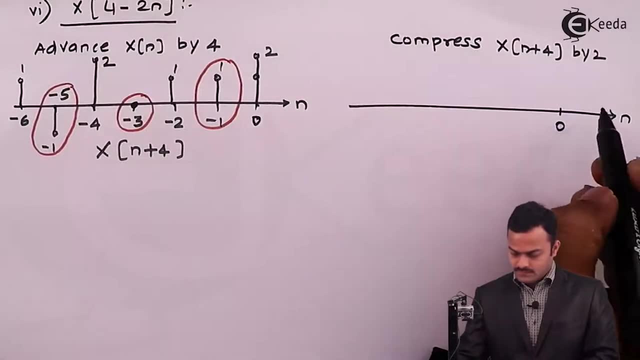 get loss. So in the end we will get a signal like this: For 0, it will be 2.. For minus 1, it will be 1.. And for minus 2, it will be 2, like this: 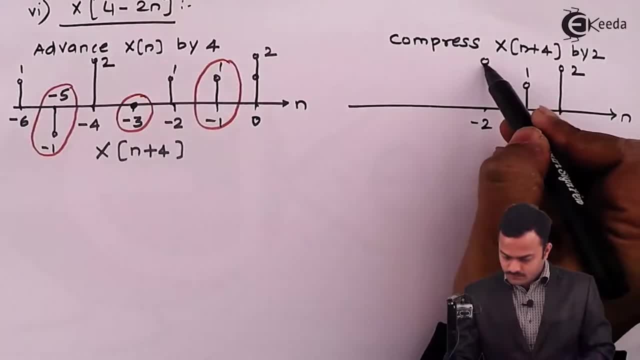 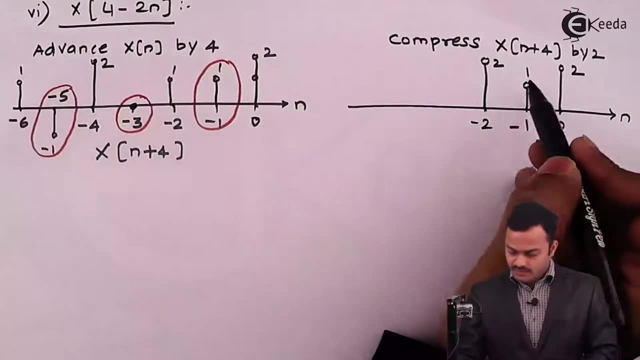 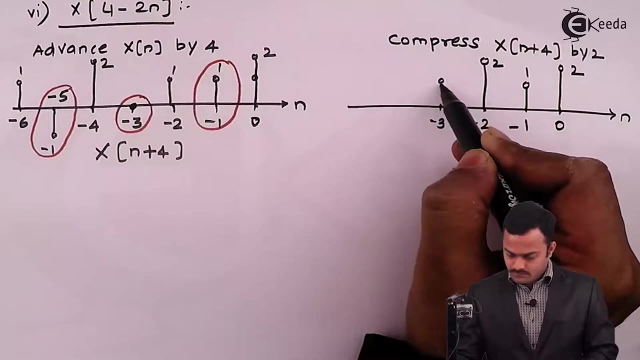 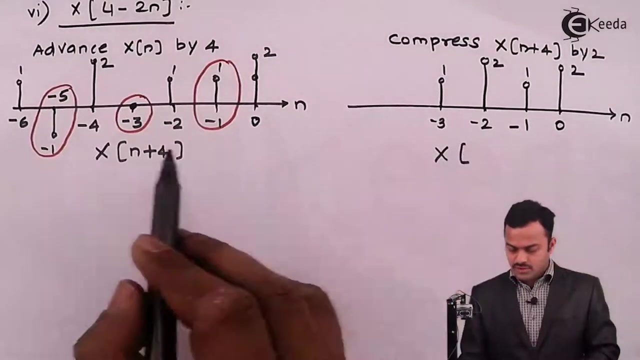 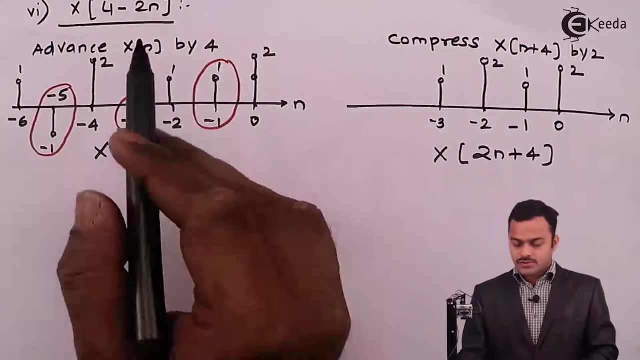 And for minus 3, it will be 1 once again. So this will be the signal, which is a compressed version of n plus 4, which is x of 2n plus 4.. Now I need to introduce minus 2n. Already 2n is present, So I need to replace n by 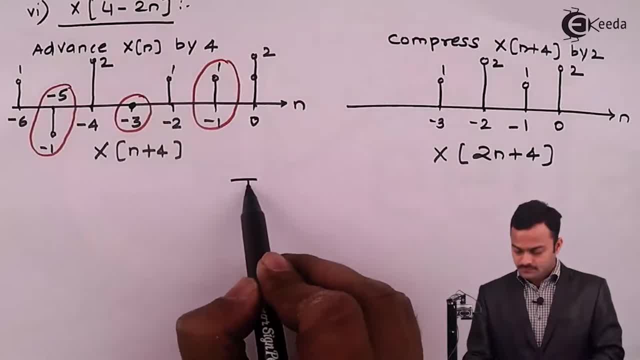 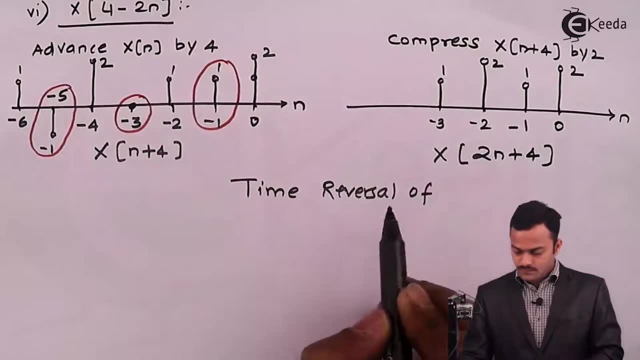 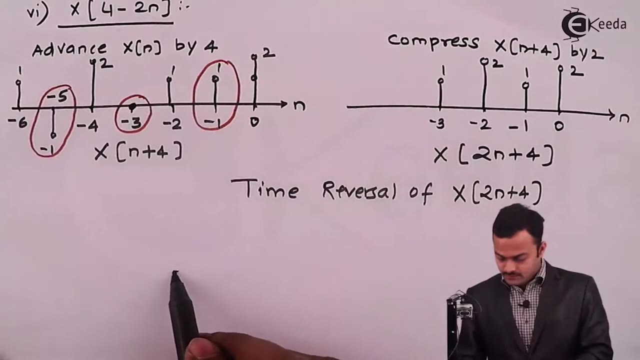 minus n, and that is nothing but time reversal. So we need to do a time reversal of x, of 2n plus 4.. So it is very simple. We will get a reflection on positive n side. So signal that we made will have a span from 0 to 3.. 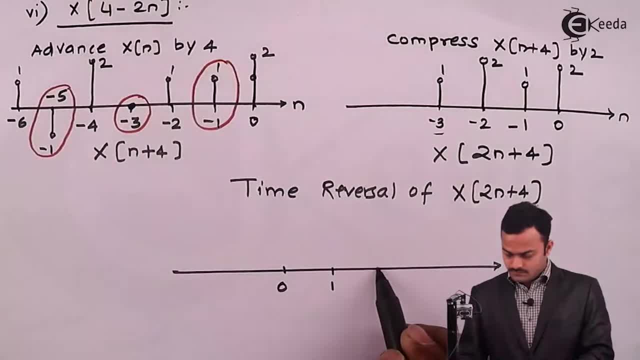 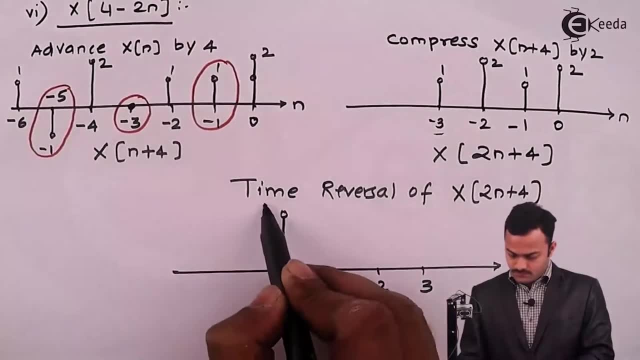 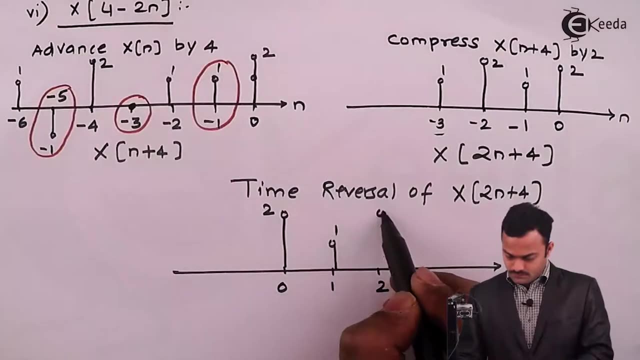 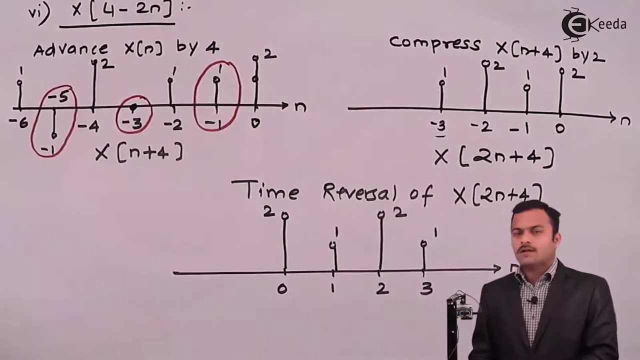 And this will be the result. Next is the wave Speed: Manual Transmission of wave Speed R to wave Speed R will also be same as previous one. We will basically have different time refrains. So here will be the've been used Limit Range phenomena And let us say for okay, this signal. 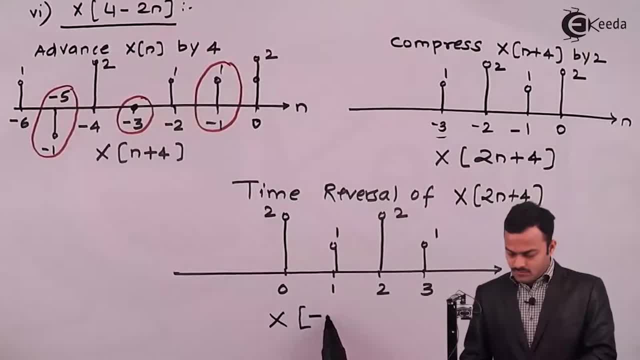 will be 0.. See when wide-slopeStop式SzZ z each area we have the times determine what we Econom 有, and this sign will have X of Minus 2n plus 4, Which we can represent as X of 4 minus 2 n. 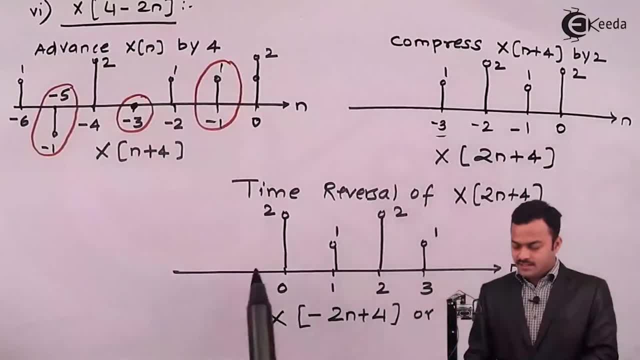 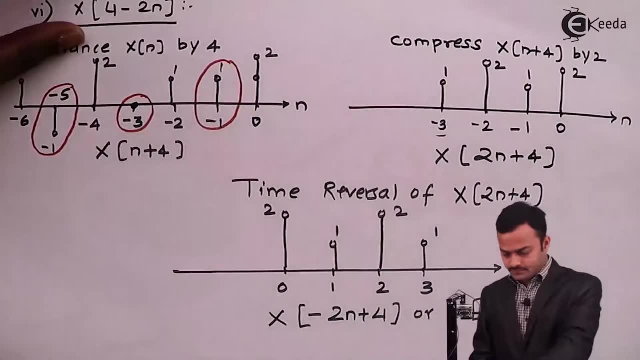 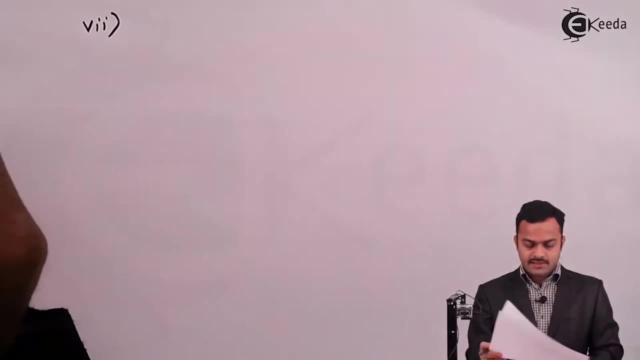 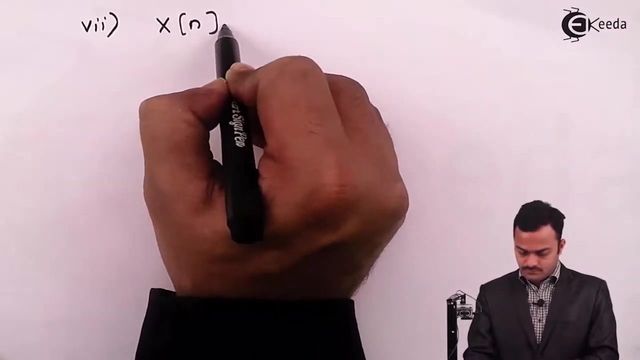 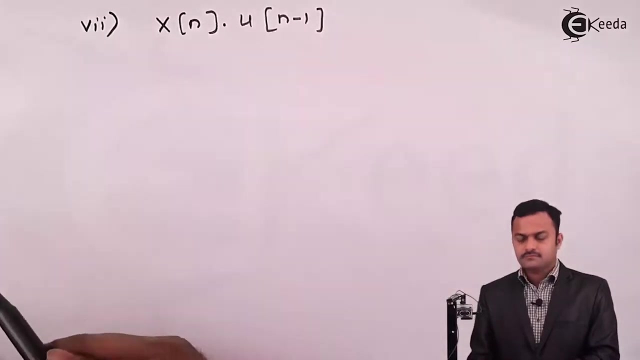 So time shifting, Time scaling and time reversal, all the three operations are covered in this signal. Let's go to the next signal. So in the 7 signal There are X of n into U of n minus 1. It's the multiplication of two signals. Okay, well, X of n, we have already plotted. 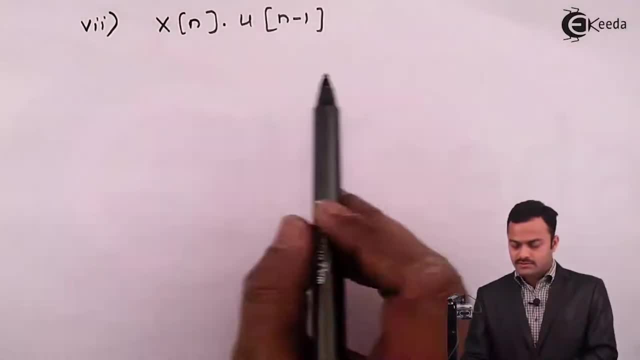 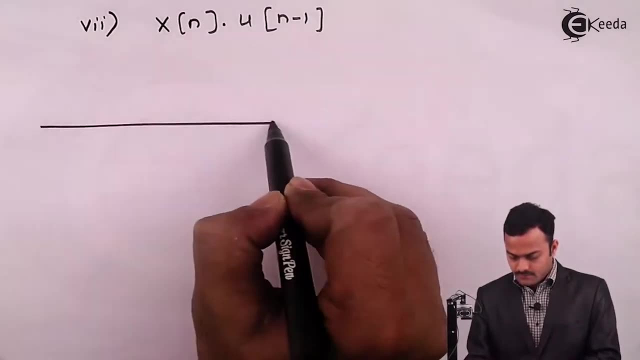 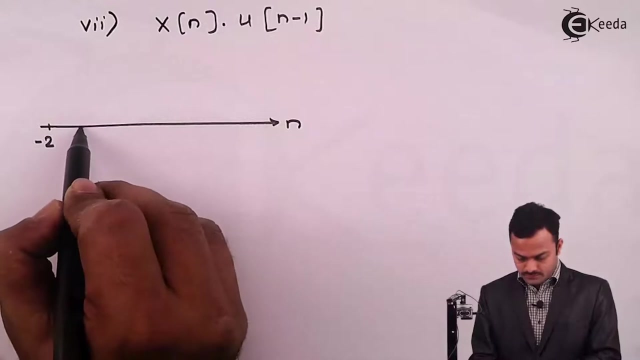 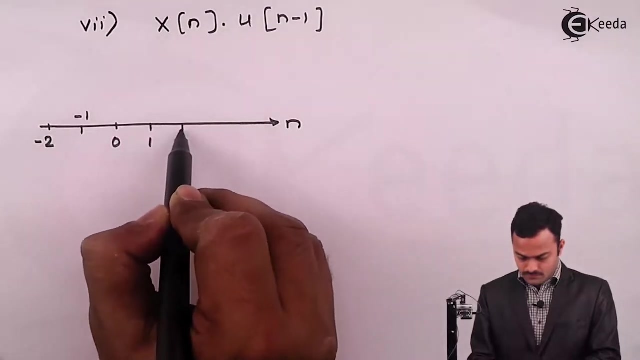 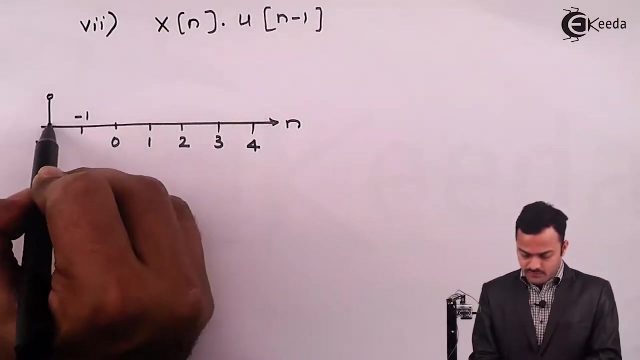 So once again we will plot, because we need both the signals on the same page so that we can find out this multiplication. So X of n. we have already plotted like this: It is having the span from minus 2 to 4, With the values ranging from 1 to 2. 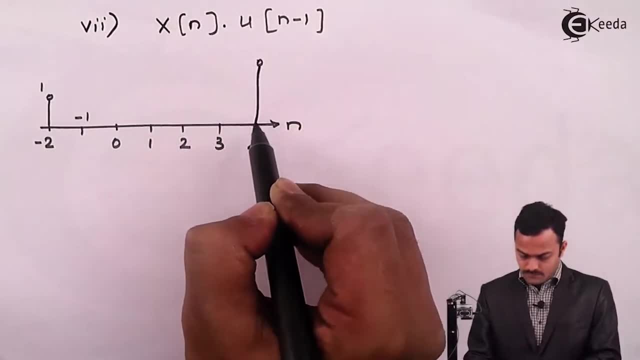 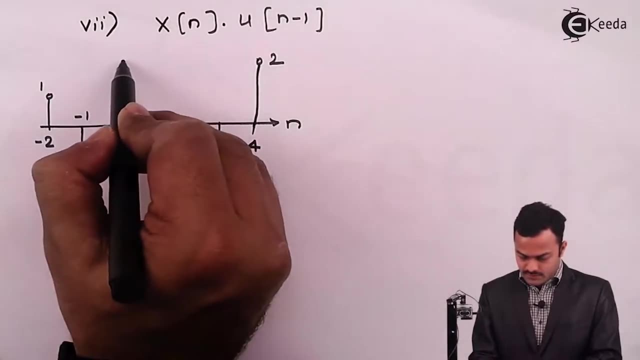 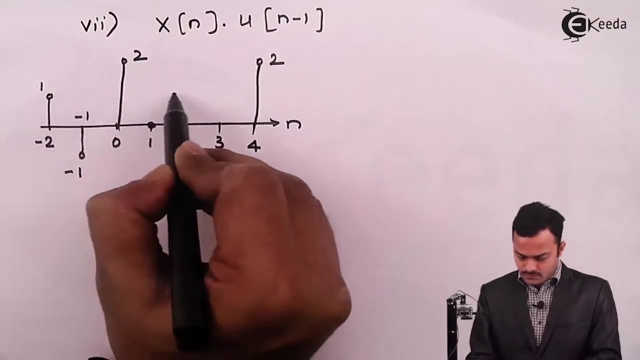 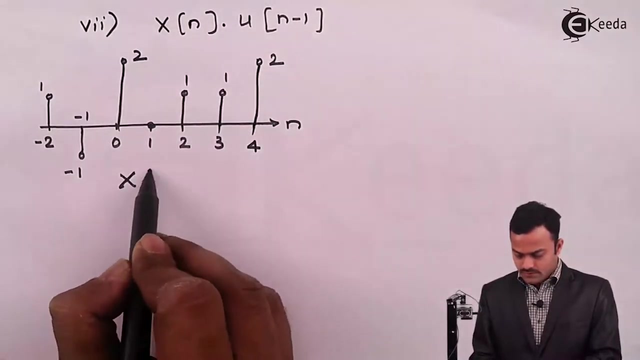 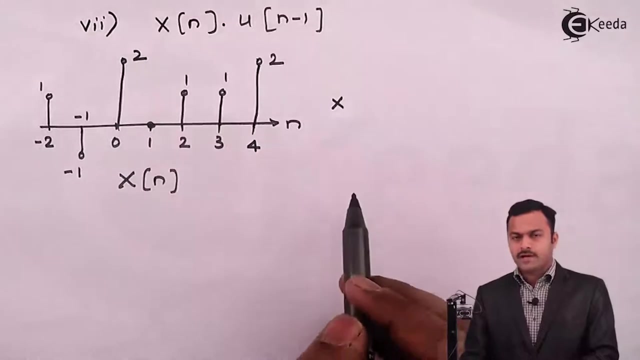 And in between it may change to minus 1. then once again we are having a 2, 0, 1 and 1, So this is X of n. We need to multiply with U of n minus 1, So U of n minus 1 is nothing but a time delayed version of U of n. 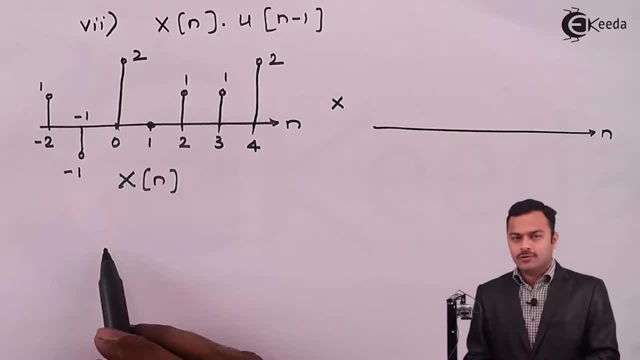 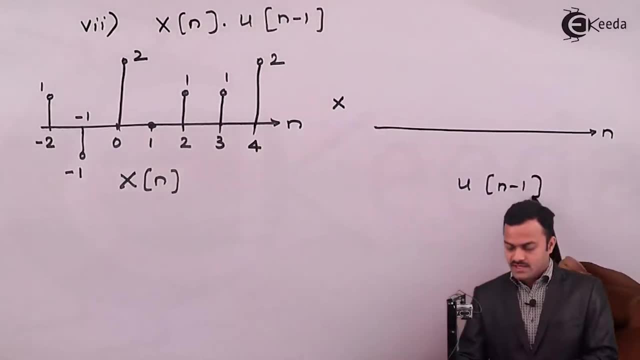 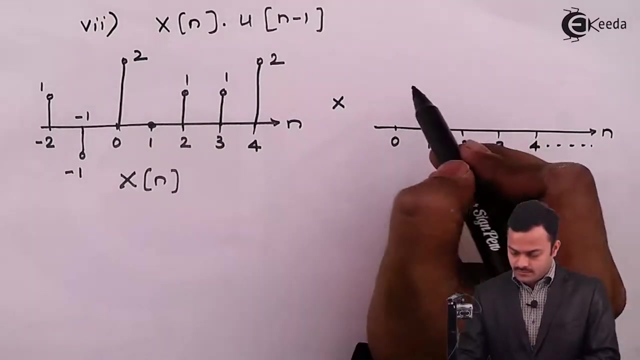 So U of n started at n equal to 0. Since I need to shift it by 1, so U of n minus 1 Will start from 1, And it can go up to Infinity. so And with the magnitude equal to 1. so every time I will get a magnitude as 1. 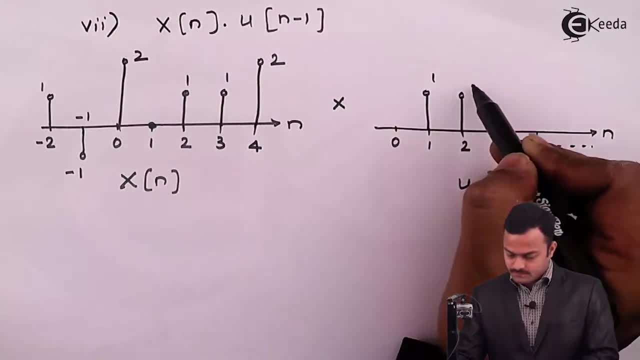 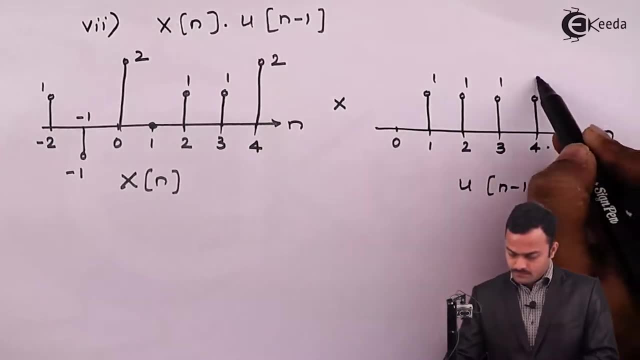 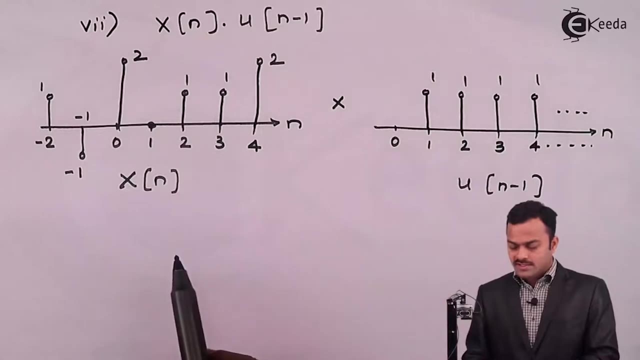 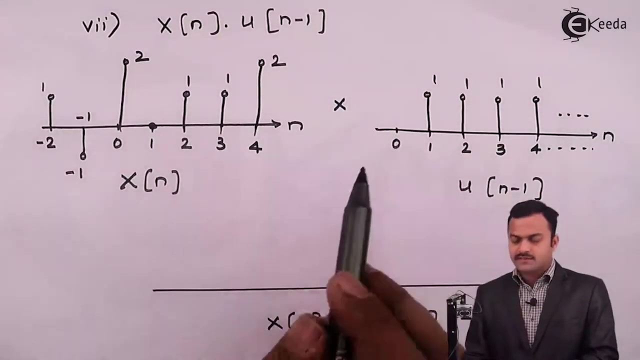 for unit step function. It will be continued. so I need to multiply these two signals. so it's quite simple because Instant by instant, I need to multiply and get answer. meaning X of n Into U of n minus 1 will be. We need to multiply the instances. for example: 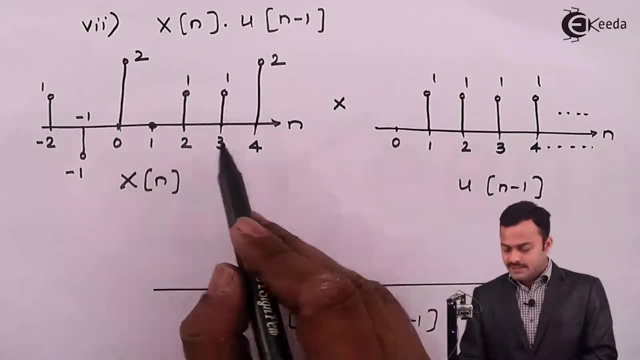 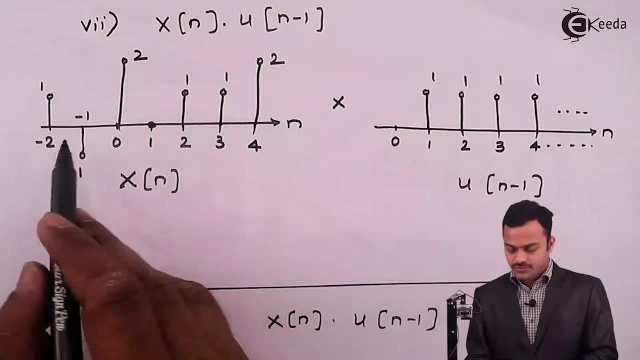 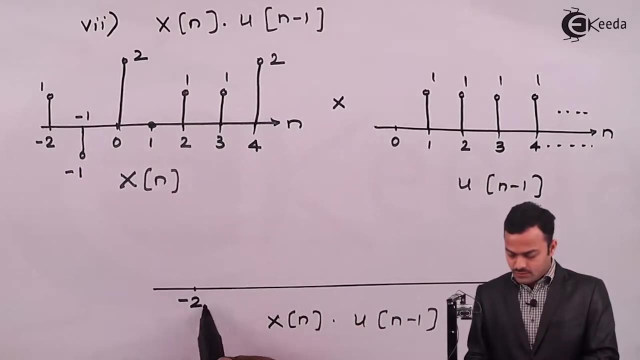 This particular signal will have the value 0, from minus infinity to 0, meaning minus 2 and minus 1 over here, getting multiplied with a 0 so that this term will vanish and in there I will not get any signal for n equal to minus 2. n equal to: 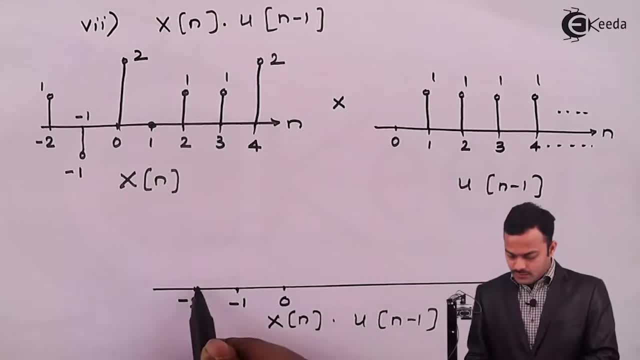 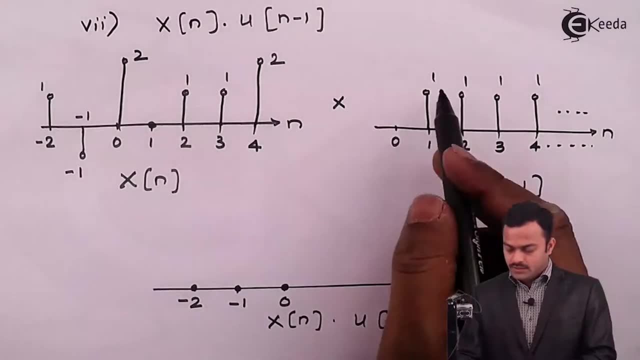 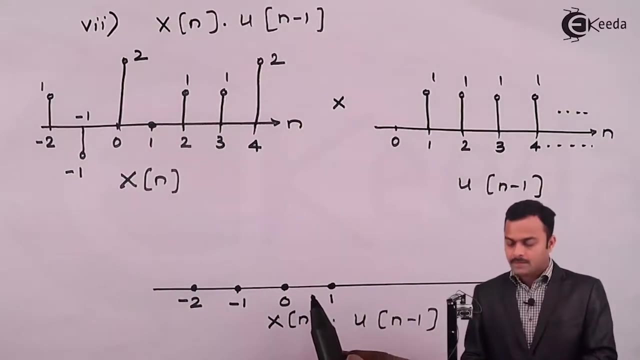 Minus 1 and n equal to 0, so 0, 0 and 0. Then for n equal to 1: here is 1, here it is 0, so once again We will get a value 0. for n equal to 1, Then n equal to 2: here It is 1 here. 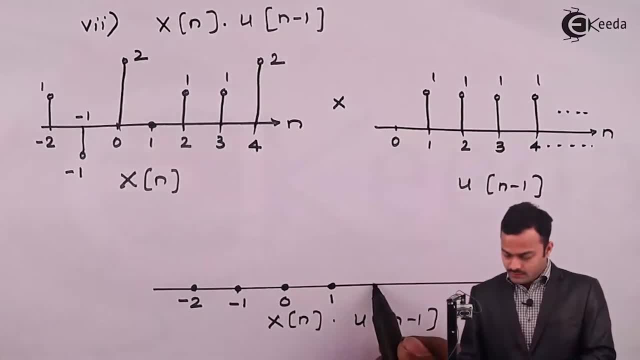 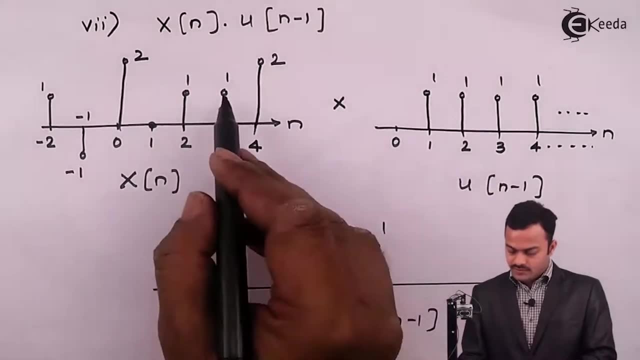 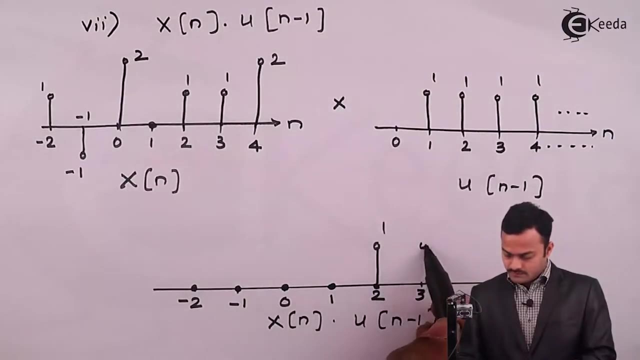 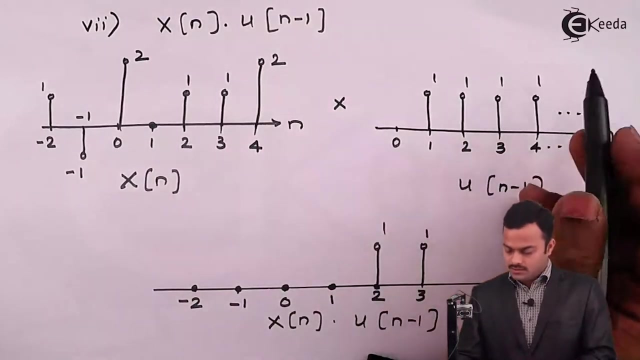 it is 1, 1 multiplied with 1. so for n equal to 2, i will get a signal equal to 1. for 3, 1 getting multiplied with 1. once again, for n equal to 3, it is 1. and finally, n equal to 4, 2 getting multiplied with the 1, answer will be 2. 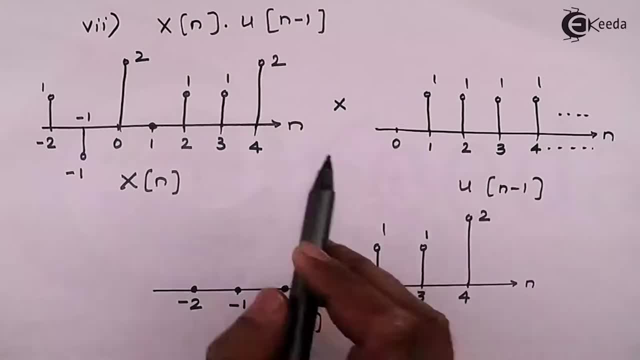 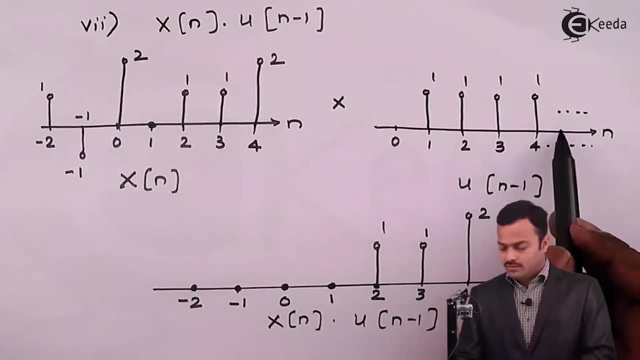 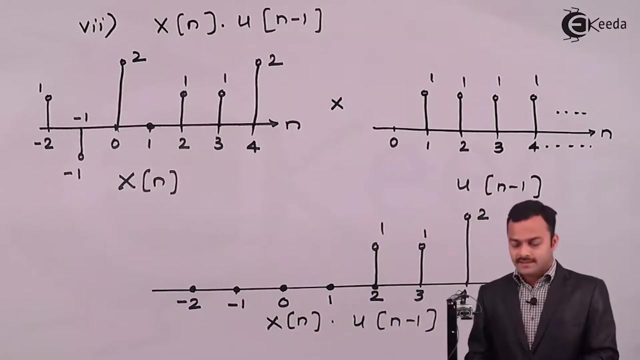 so 4 onwards, x of n is having the value 0. so 0 is getting multiplied with the 1, because 4 onwards this will have the value 1. so in the end 4 onwards signal will have the values 0 till infinity. so this is a signal which is x of n into u of n minus 1. let's go to the next signal. 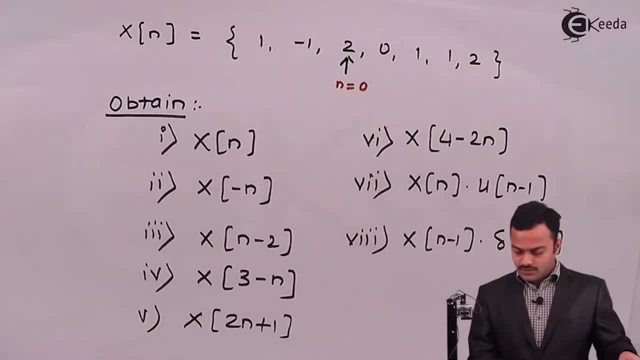 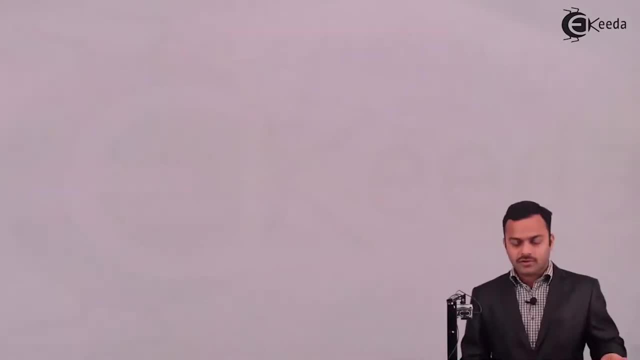 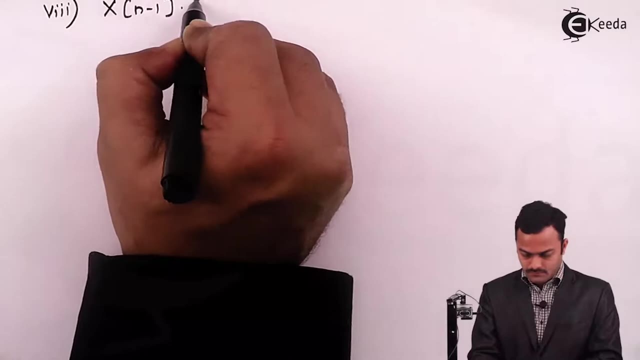 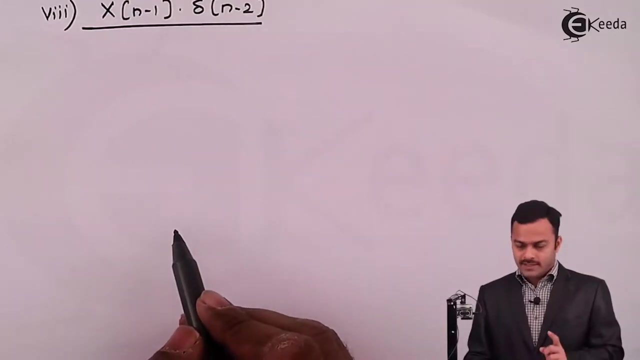 so here it is x of n minus 1 into delta n minus 2. so let's first plot x of n minus 1. before plotting n minus 1, let's plot x of n once again, so that right from the start we can show how this particular signal can be obtained. so 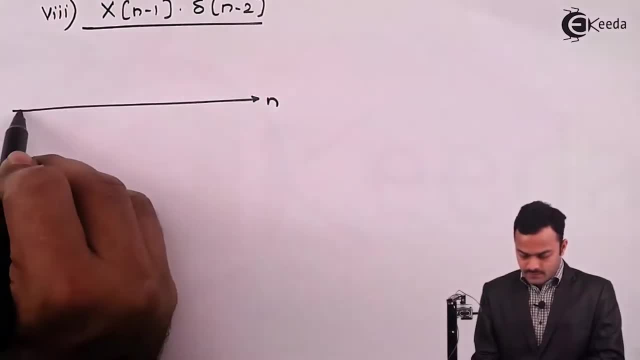 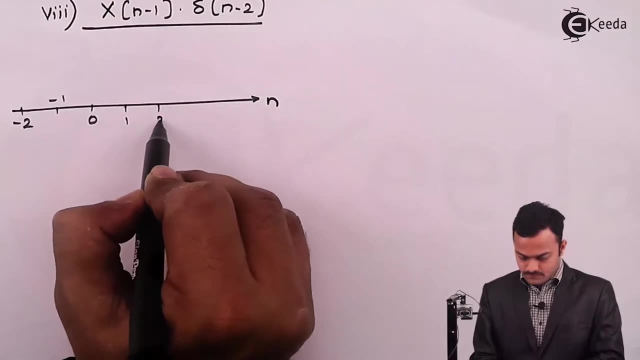 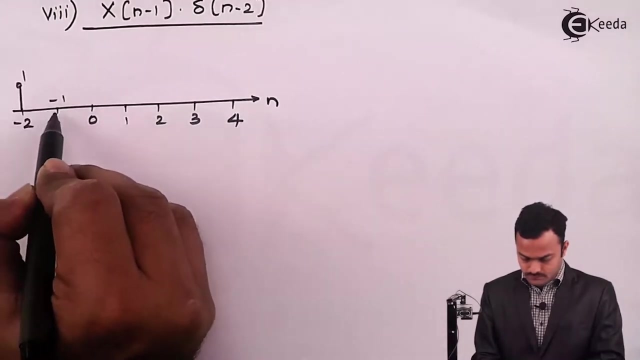 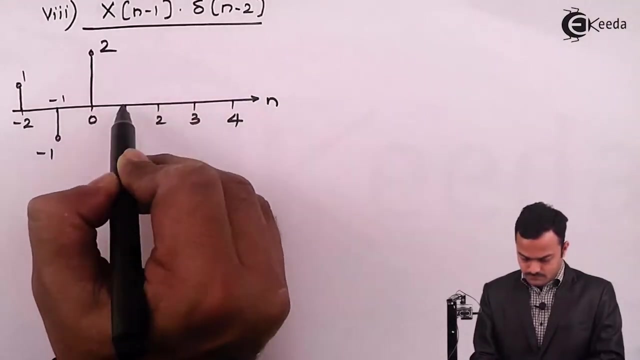 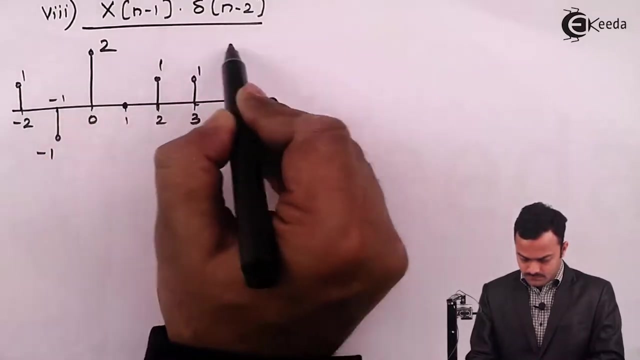 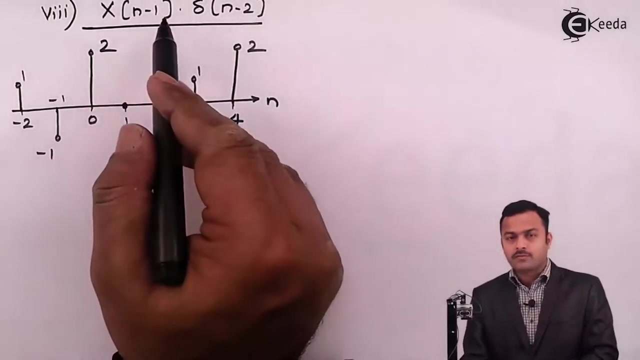 let's quickly draw x of n. let's try this strategy. so all this calls x of n. we have to ink x of n minus 1, some other forgot perspective when you viewers need x of n. until we want to get this expression, whether x of n is equal to 1. 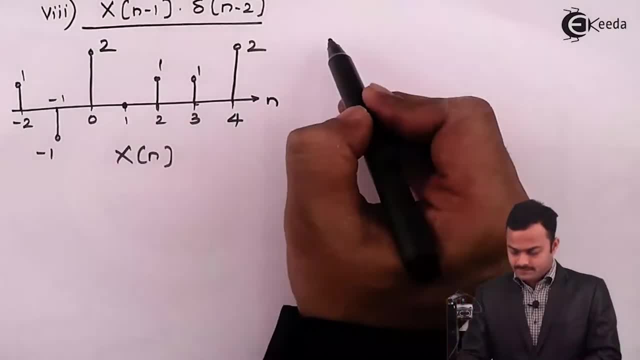 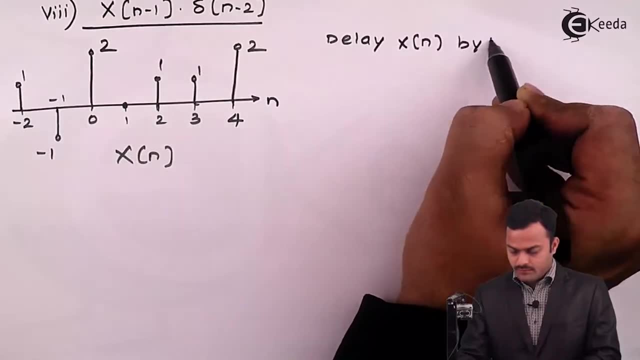 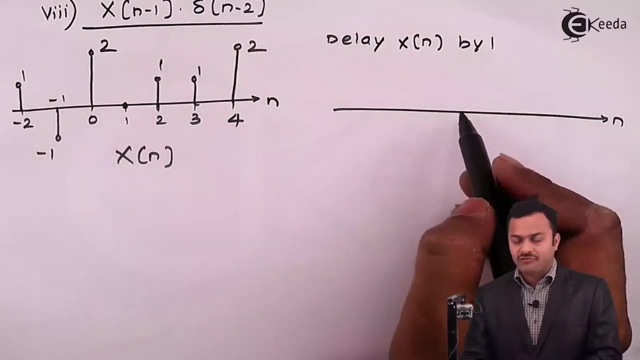 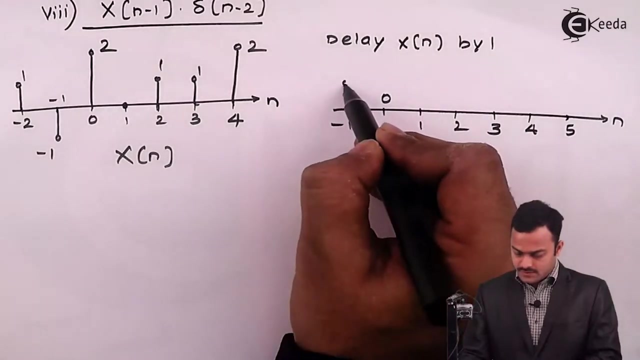 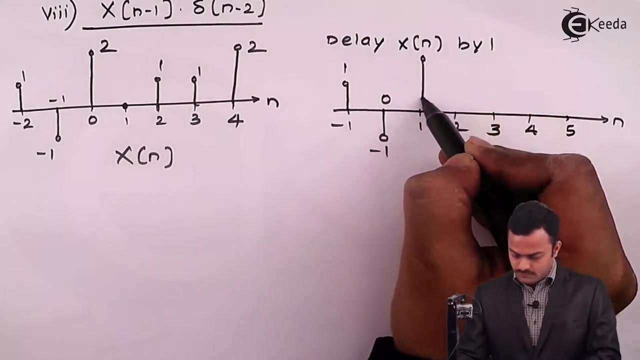 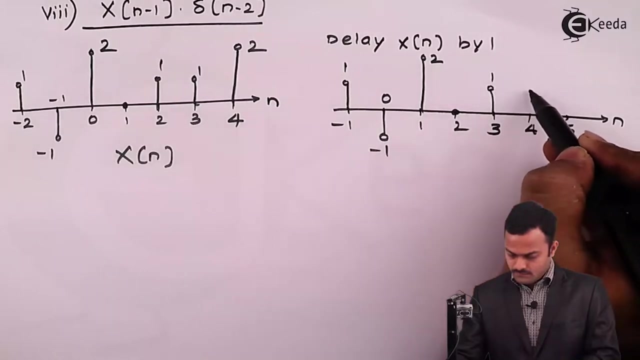 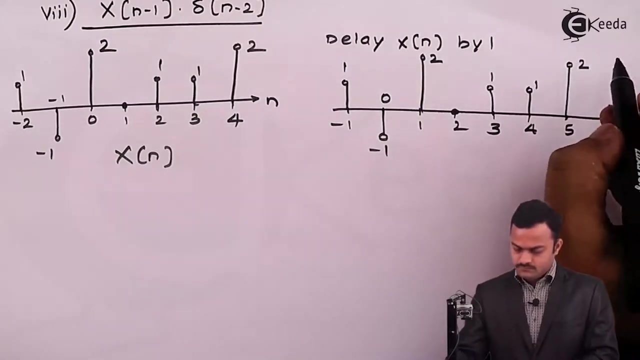 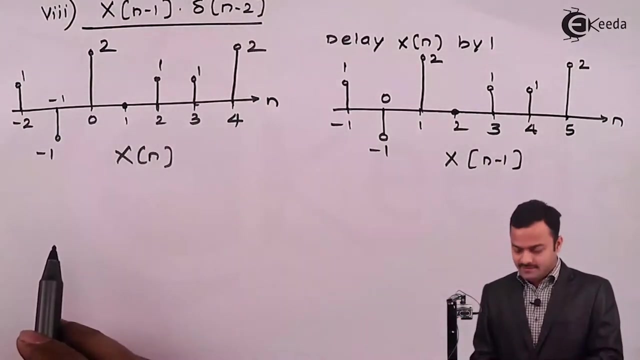 delay of X of n. so if we delay X of n by 1, we will get a span of the signal from minus 1 to 5 with the values like this: so this is X of n minus 1. now we need to define what is delta. so before writing, delta n minus. 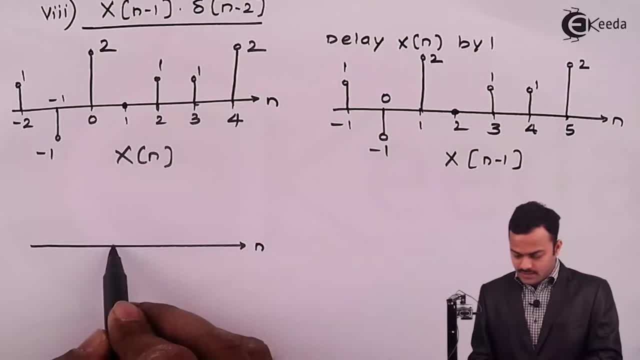 2 delta will be like this: it will have the value equal to 1 only for n equal to 0. remaining points it will not have the value equal to 1. so this is X of n minus 1. so this is X of n minus 1. it will not have any value meaning for 1, 2 up to infinity, minus 1 minus 2 minus. 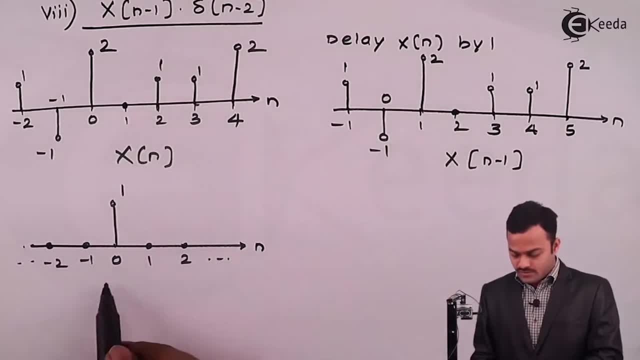 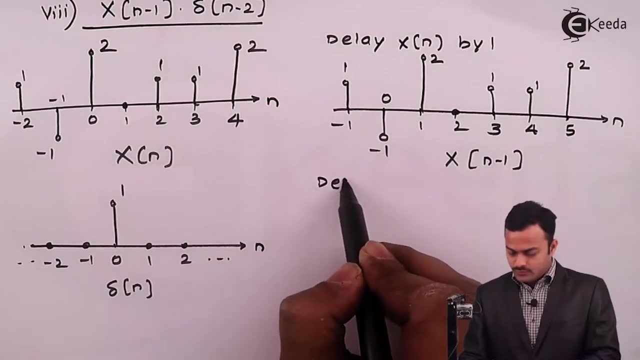 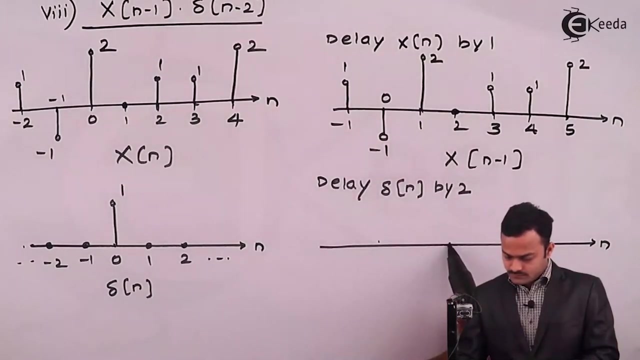 infinity, it will be 0. so this is a delta n. what do we want? delta n minus 2. so we need to delay this by 2. so if I delay this by 2, we will get a signal like this: for a sparse interval, go to delta n minus 2 and choose. 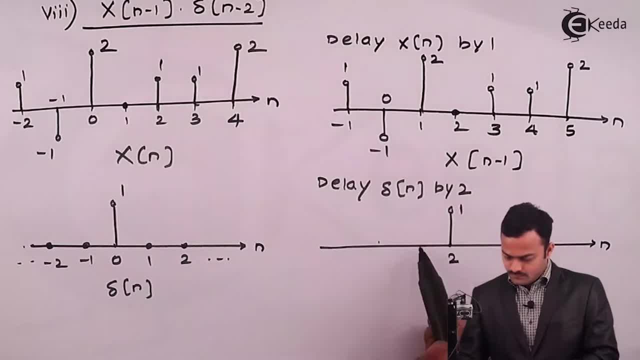 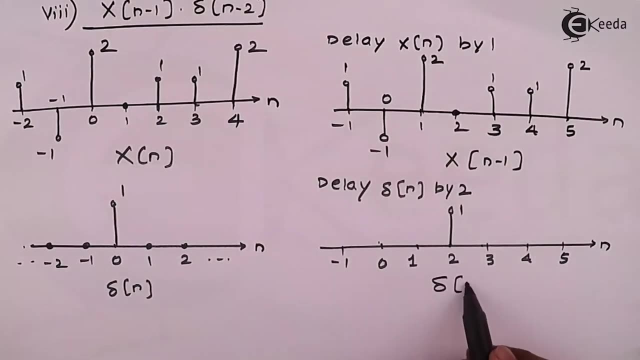 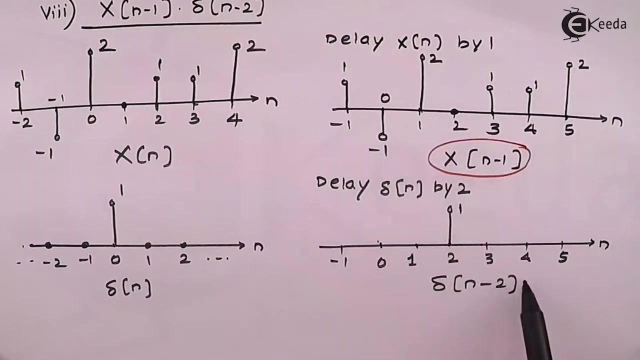 crosstalk for remaining intervals. А deputy hat will have the value 0, like this. so this is ι delta n minus2. now our job is to multiply X of n minus1 with delta n minus 2, instant by instant, and if you see over here for all the points from minus 1 to 5, or you can take: 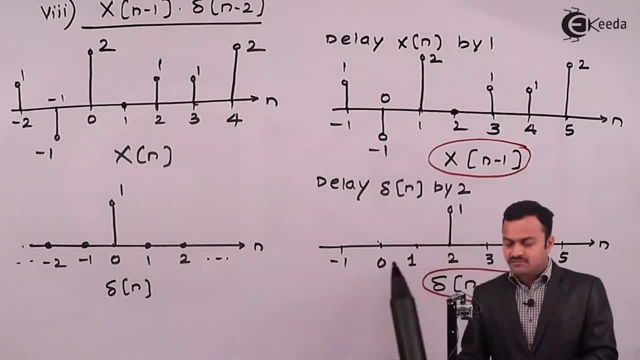 from minus infinity to infinity, we will get a signal which is nothing but a 0. so every time either of element is 0, so in the end, what we can say, the signal which is a multiplication of these two, can be shown just like this: no element.